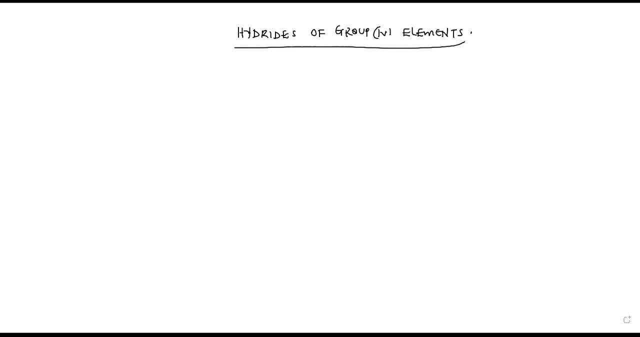 Okay. When we say a hydride, of course we need to first understand what a hydride is. When we say a hydride, we are trying to look at a compound of hydrogen with a metal, A binary compound of hydrogen. 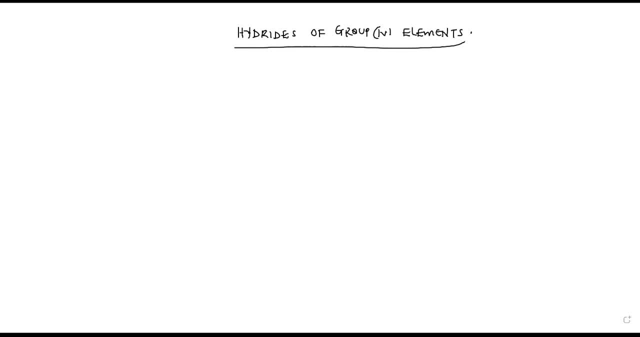 with a metal, meaning that we form hydrides of compound by combining a metal and then hydrogen. So, for example, we have got the formulas of hydrides of group four elements. Then we have, for example, the formula of the hydride. We've got CH4 and this is methane. 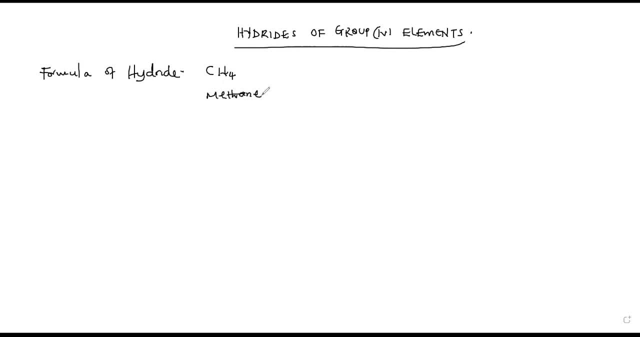 So the hydride formed by carbon is methane, CH4.. We've got SiH4, people call it silicon hydride, but we call it silane Silane. We've got what we call germanium hydride, but its real name is germane. 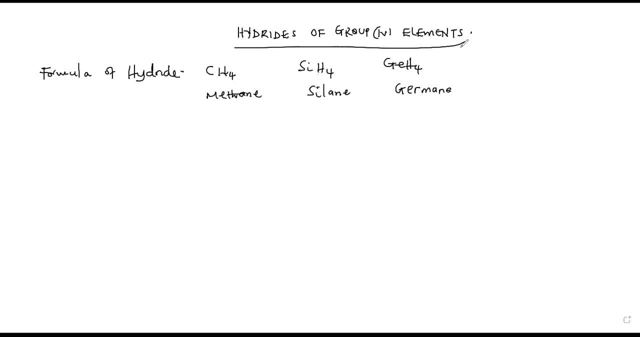 We've got what we call tin hydride, but its real name is stanane- What do you call lead hydride? And its name is plambene. So these are hydrides formed by group four elements. 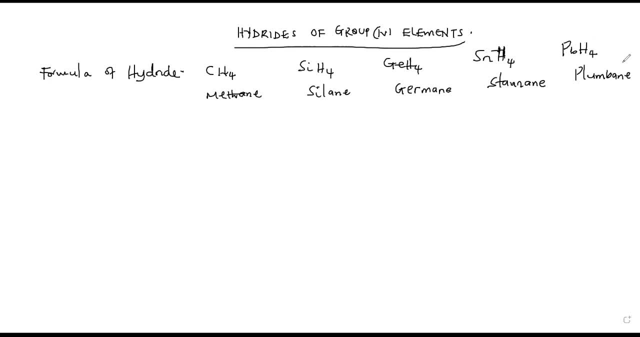 In other words, these group four elements combine with hydrogen from hydrides. okay, So a binary compound of an element with hydrogen, that is the word metal. but all these ones may not be metals. okay, They are not metals. that is what we need to know. but basically that is what we are. 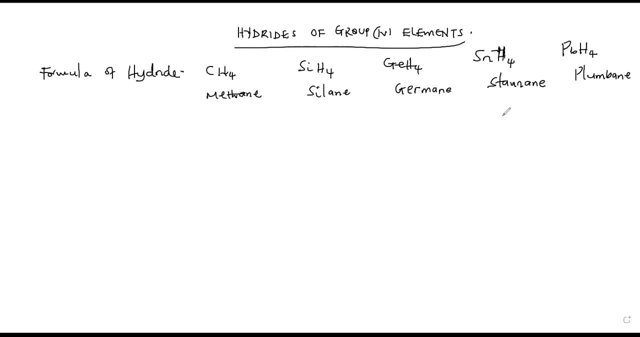 having. Carbon is a metal, as we said. silicon, germanium are metalloids and tin, lead are metal. okay So, but each one combined with hydrogen to form a hydride. All these hydrides, all these hydrides. 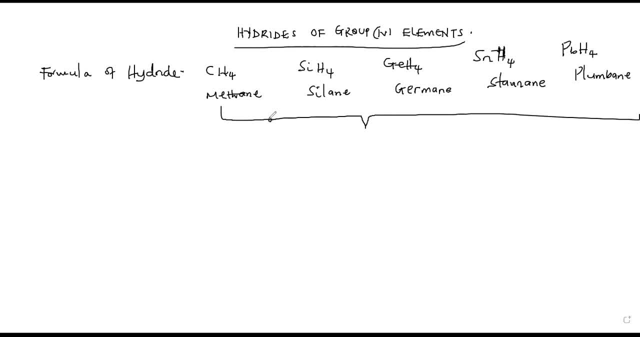 They are metals, They take on gaseous physical state. So all of them are gases, So they are gaseous in nature, so they take the gaseous physical state. Then still, all of them are covalent. that is the bonding. they are covalent, they take. 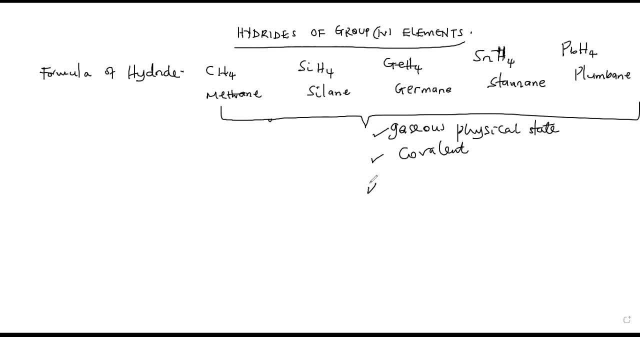 on covalent bonding. And then they are by structure. they are simple, molecular. They are simple, Simple molecular And because of the number of hydrides and their nature, you can see that they are tetrahedral. They are tetrahedral, all right. 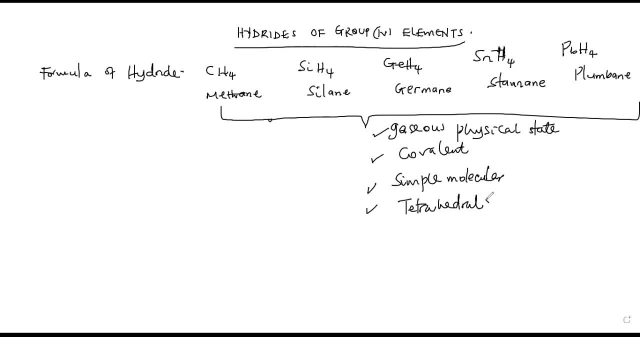 They are tetrahedral And you still see that now, that is the shape, the agassias in nature, that is the physical state, or the agassias they take on covalent bonding. their structures are simple, molecular and their shapes are at a trahedron. 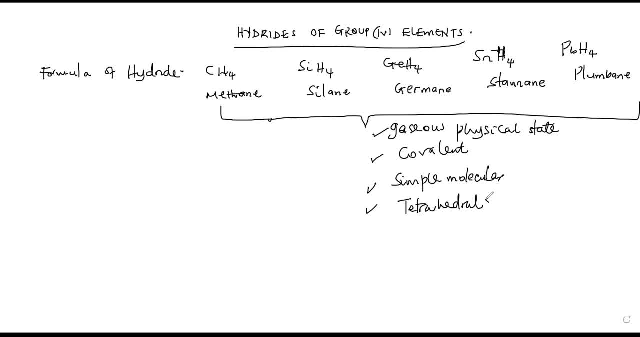 now, of course, we've said that, bonding wise, they all form hydrides with a simple molecular structure and tetrahedron, and they are all colorless. so that is what we need to know. but how do we form them? how do we form these hydrides? 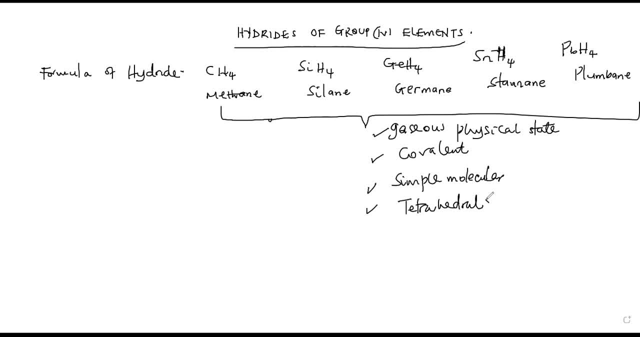 because the question can come specific when they want you to describe how these hydrides are formed. they may want you to describe how these hydrides are formed, so let's see how these hydrides are formed. formation of group 4 hydrides. 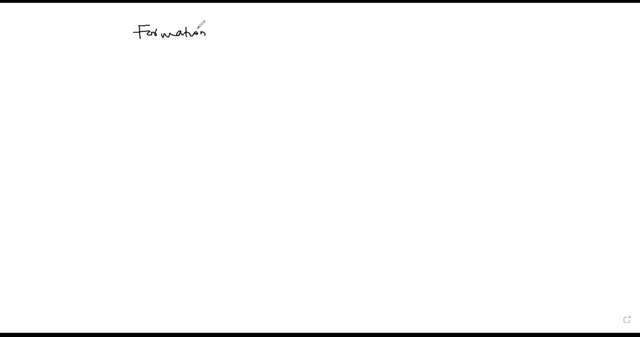 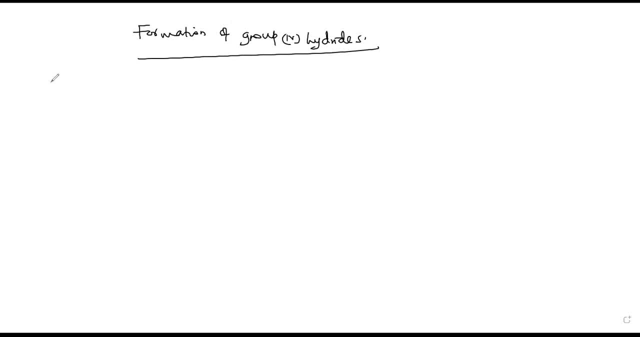 is to describe how the hydrides of group 4 elements are formed. how the hydrides of group 4 elements are formed, one would begin with Rider, with methane, methane, us. we can idealize the carbides, uh, the carbide of beryllium. 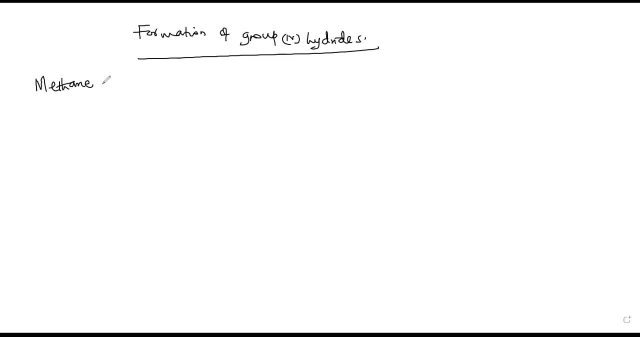 and the carbide of aluminium. So methane is formed by hydrolysis of beryllium carbide, And let's consider all aluminium carbide, beryllium carbide or aluminium carbide. So So Now, from these carbides, the hydrolysis can lead to the formation. 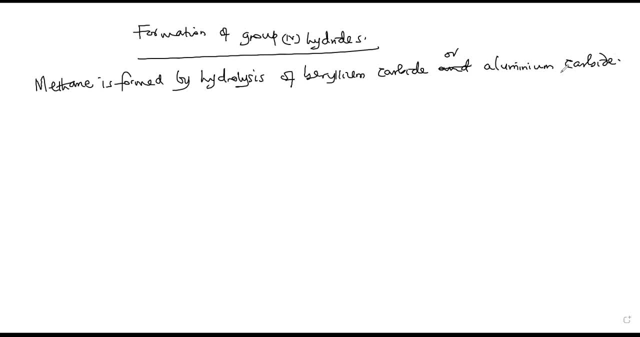 The hydrolysis of these carbides can lead to the formation of the hydrates that we're interested in, For example. For example, if you have aluminium carbide, Okay, When we say it hydrolyzes, It means that the carbide is combining with it, with water. 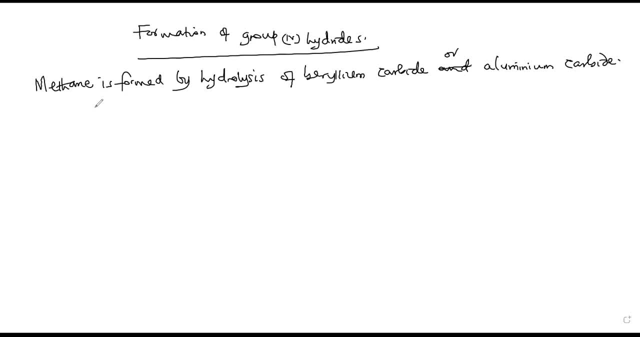 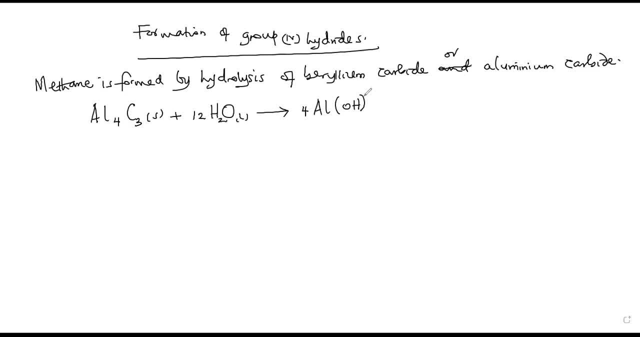 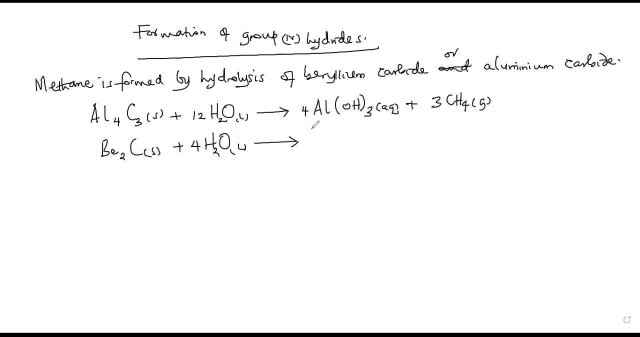 Or is it to do too much of you is to do too much of uh is to do too much of practice. so you're from beryllium hydroxide and methane gas. so that is how we form methane gas. then we need to also know: 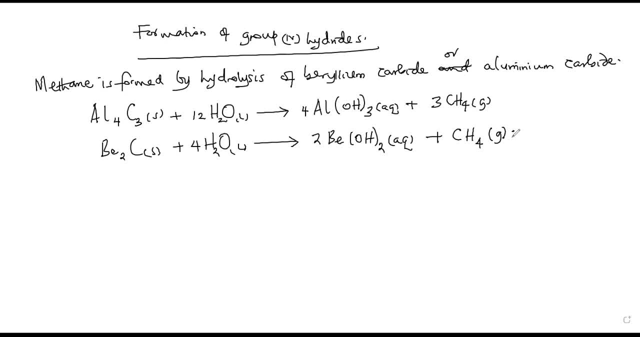 how other hydrates are formed. okay, the hydrate is left is, uh, the silane we are left with the silane we are left with. so how are they formed, those ones? the rest are formed by reducing tetrachlorides using a reducing agent of lithium, aluminium tetrahydrate. 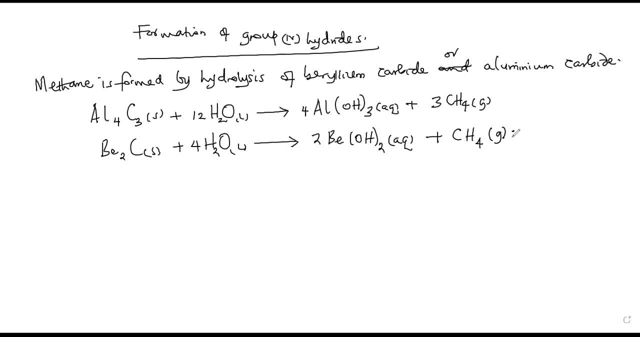 in presence of dry ether. okay, so we can say: maybe silane, gemene, stannane and plambene are formed by reduction of their corresponding tetrachlorides by lithium ammonium hydrogen nitride in presence of dry ether. one can call it lithium tetrahydridoaluminate. but you can take this, one can add, under condition of temperature. but even if you say by reducing, by using lithium- aluminum hydrate in presence of dry ether, one can call it lithium tetrahydroaluminate. but you can take this, one can add under conditional temperature. but even if you say by reducing by using lithium- aluminium hydrate in presence of dry ether, one can add on the condition of temperature. 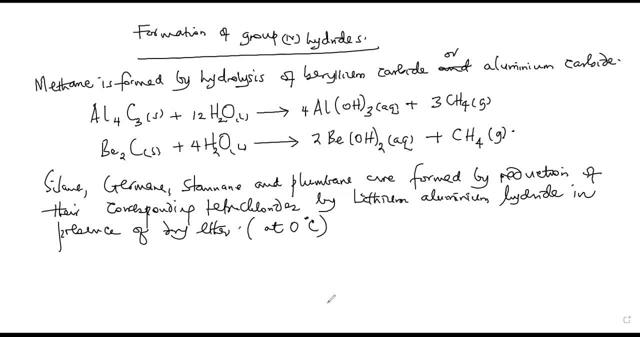 but even if you say by reducing, by using lithium aluminium hydride in place of dry, that is enough. so it means that if we need a silane, we shall have silicon tetrachloride liquid. you add lithium aluminium hydride and it's a solid. you form silane. 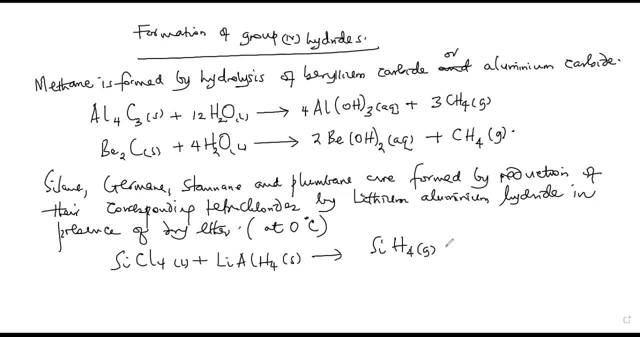 gas. all of them are gases plus lithium chloride solid and then aluminium chloride solid. the same applies to others. when you get germanium chloride, reduce it with the lithium aluminium hydride. you form germanium hydride, or what we call jomaine gas plus lithium chloride. 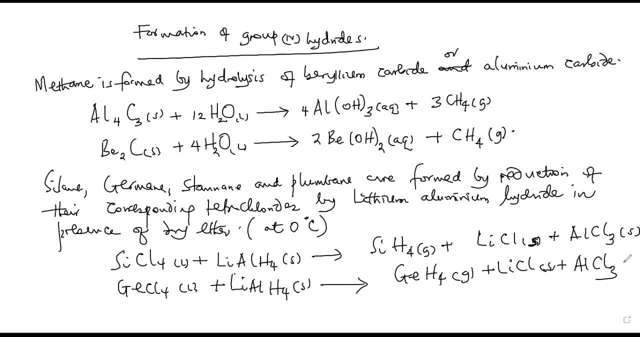 solid, then plus aluminium chloride. sorry, if you get tin folclorel, aluminium chloride solid. if you get tin folclorel, you add lithium aluminium hydride, so it will form stannane, which is tin hydride plus lithium chloride plus aluminium chloride. sorry. finally, if you want prambane, you'll get. 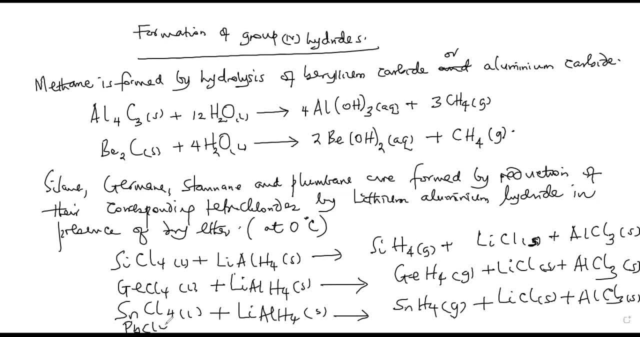 lead tetrachloride plus lithium aluminium hydride, you form your prambane plus lithium chloride plus aluminium chloride. it is Cl3 at the end, which is sorry. so this is how easy we can form the group four hydrides. interesting. now of course we need to know other physical parameters, okay. 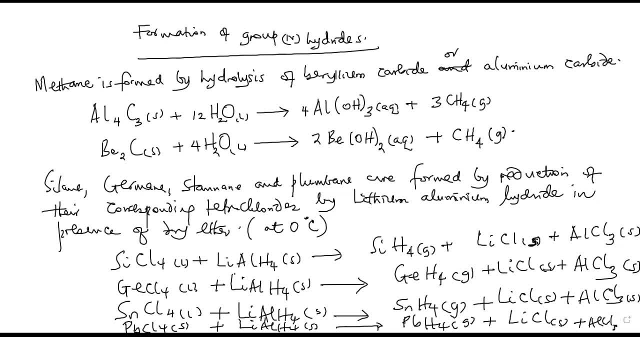 we need to know the physical parameters that these hydrides undergo, and among those physical parameters you're going to look at the, the melting point, okay, and then the stability of these hydrides. then after, maybe after looking at some reactions, okay, then we shall. we shall look at a question that appeared in an exam of last year's UNEBL. 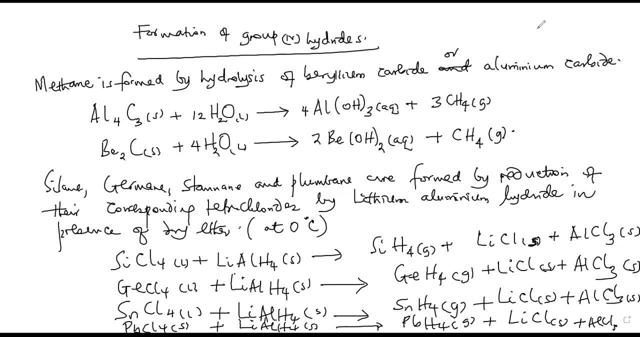 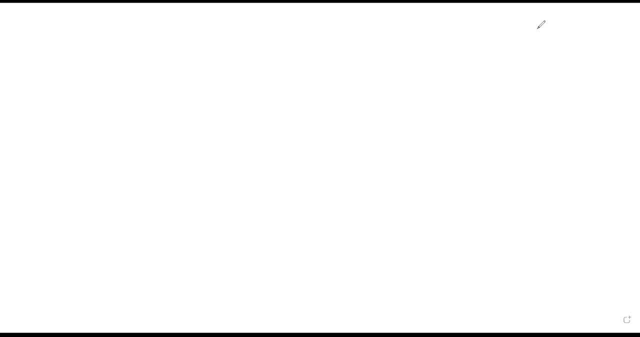 right. so let's go ahead now to look at the melting points. so, of course, if we have a hydrolysis and we have gotten some more Clear Point, and then we are given the boiling point, which is, in degrees, silicious, I've always, in all my work, I've always described to you how we explain our trends. 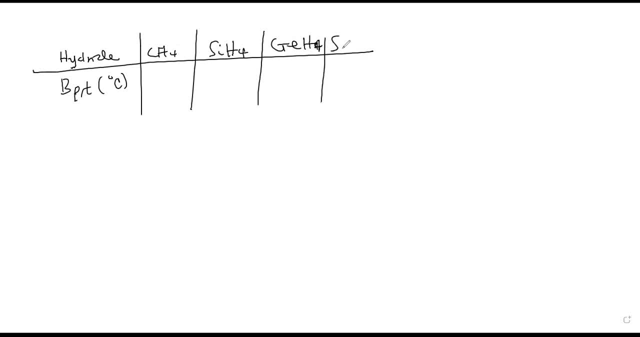 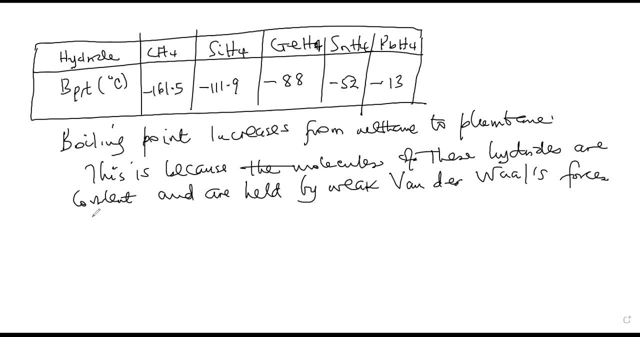 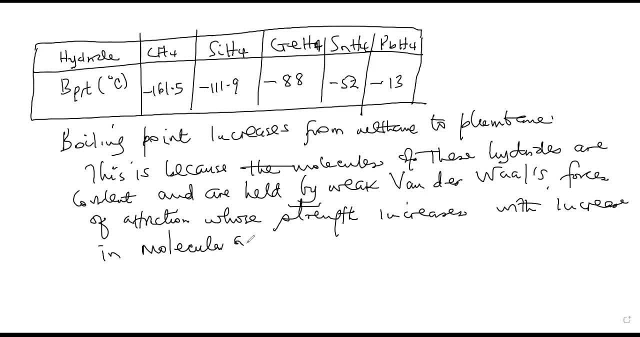 size and weight in molecular size and weight. All right, So basically this is how it is doing. Molecules of these hydrides are covalent and are held by weak vandal forces of attraction, whose strength increases with increase in molecular size and molecular weight. 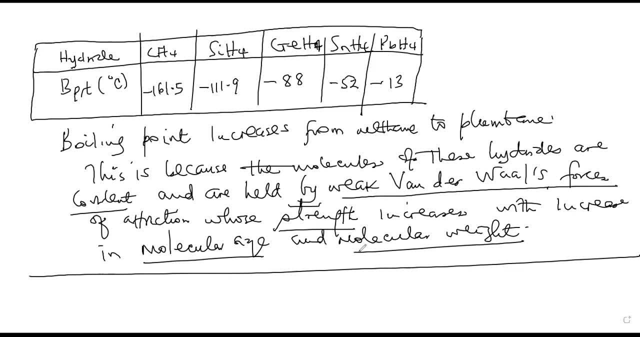 As simple as that. So this one explains how the trend increases. All right, Then from there, decompositions, okay, decomposition temperature of these hydrides. we can also be given a trend where we have to explain the decomposition temperatures or the stability. 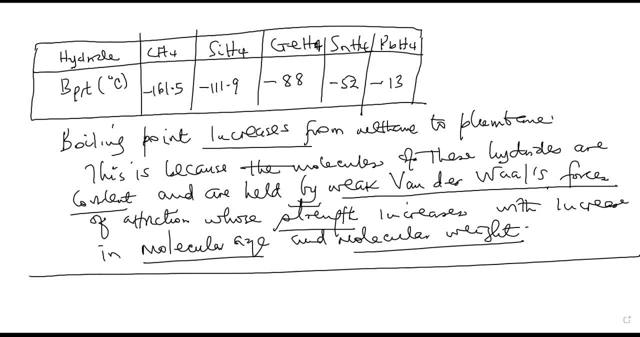 the trend of thermostability of these hydrides. So let's say the trend of thermostability of these hydrides. So let's say the trend of thermostability of these hydrides. So let's say the trend of thermostability of these hydrides. 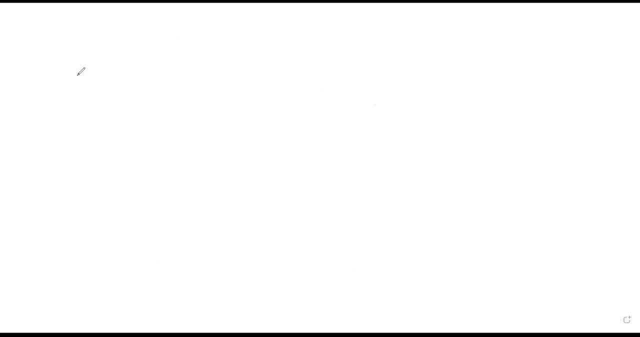 So let me also talk about that. So let me also talk about that. In this case, you're given a hydride and a decomposition temperature. What a temperature it requires to decompose The hydride is given. we have methane. 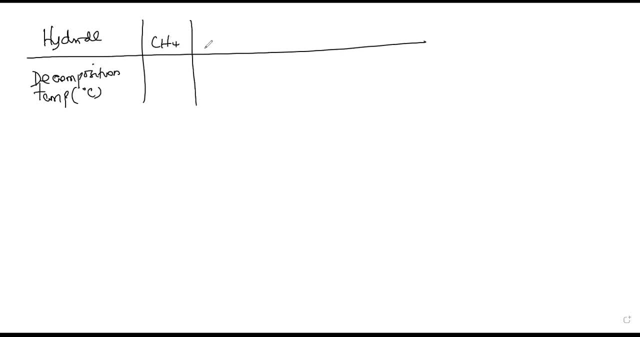 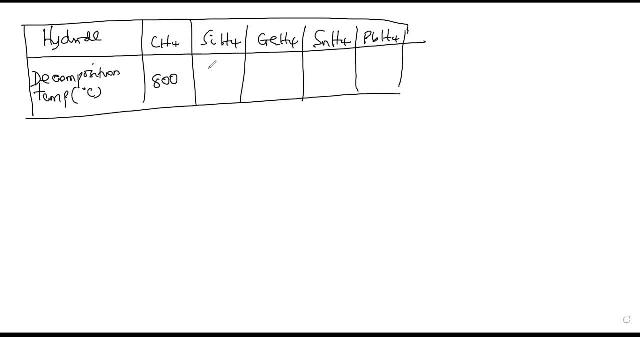 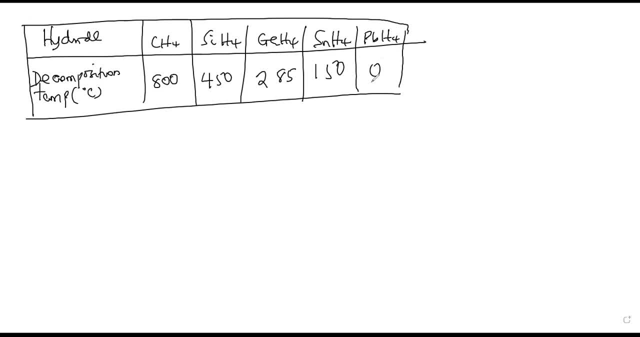 And for plambin zero. So they can ask you to explain the trend in thermostability, The trend in thermostability of the hydrides, The trend in thermostability Of course. you can see that first of all. 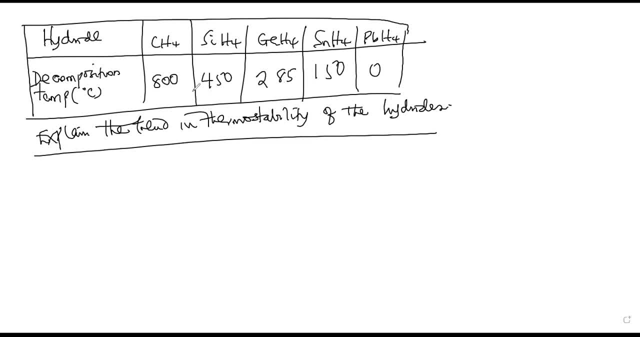 the decomposition temperature is decreasing from methane to plambin. meaning that the decomposition temperature is decreasing from methane to plambin. meaning that the if the temperature required for it to decompose is decreasing, then the thermostability also decreases. Okay. 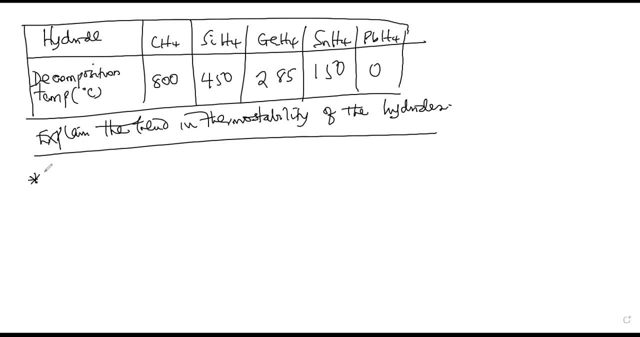 It would be better if one starts by saying decomposition temperature, though they want us to talk about the thermostability, but the thermostability is as a result of the composition temperature. Composition temperature decreases from methane to bromine, Therefore thermostability. 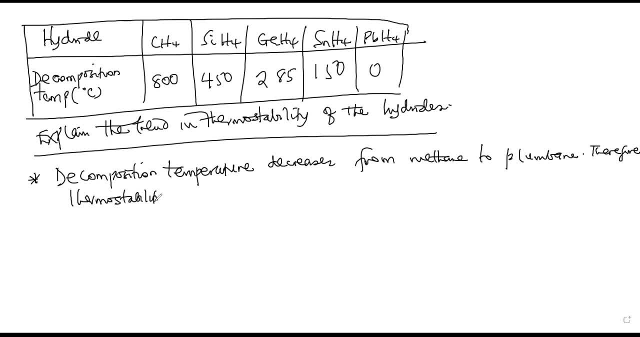 decreases from. also decreases from methane to bromine. Decreases from methane to bromine. When we are looking at all compounds, the tetrachlorides, the dioxides, the monoxide, we looked at the aspect of thermostability. 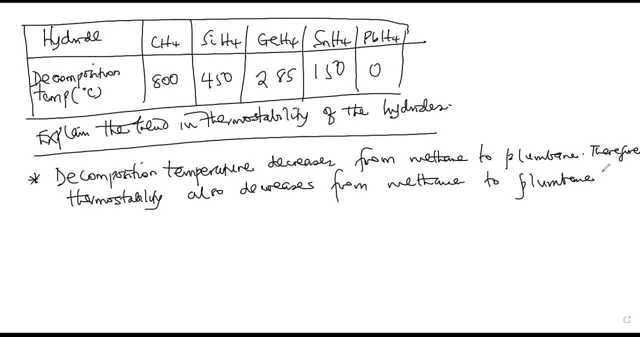 However, in some cases we are looking at it fluctuating like for dioxides, But now for this case, the decompression temperature decreases from methane to bromine And therefore also the thermostability decreases. What brings about that? 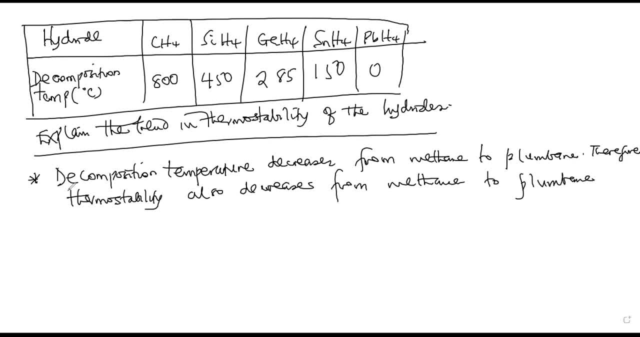 We know that from carbon to iron, it is ready for iron- The ionic radius increases, And when the ionic radius increases- okay, the bond length decreases. And when the bond length decreases, it means that the bond is becoming short but strong. 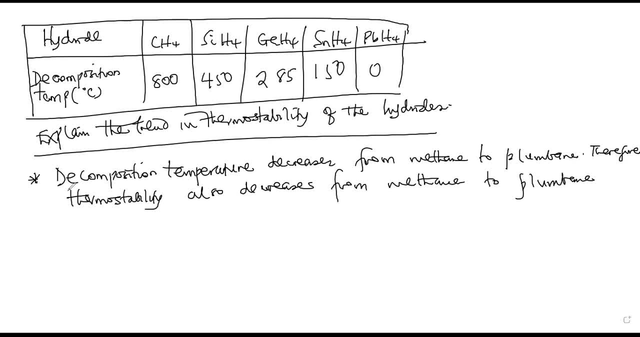 When the bond is becoming short but strong, then it becomes hard for it to be broken. Okay, Because the stronger the bond, the harder. the harder. the harder it takes to be broken. Okay, The cationic size increases from carbon to iron. 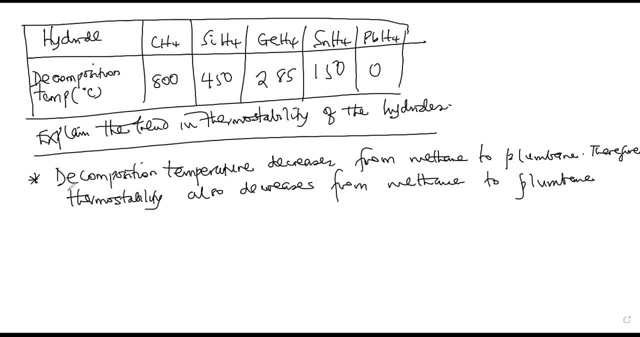 to iron, Meaning the elementary hydrogen bond. The cationic size increases from one element to another, Rather from carbon to iron to ready for iron. It also means that because the bond length increases, the cationic size increases. Sorry, I beg your pardon. 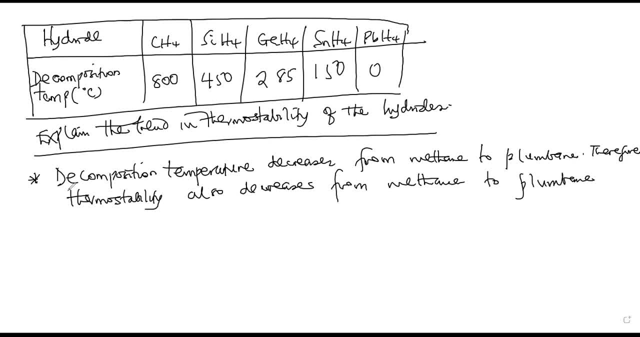 The cationic size increases from one element to another, Or rather to ready for iron. when the cationic radius increases, it means that the bond length increases. the element hydrogen or the element hydrogen bond length increases. and when the bond length increases, it means that you have a longer bond. 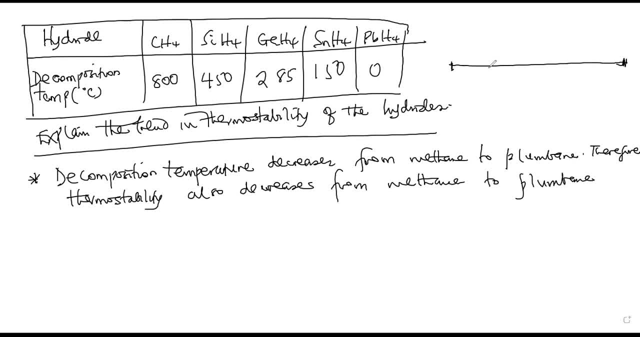 when the bond is long, then it is weak because you can touch here, like, and you break it within. but if the bond is short, it is strong because it's very hard to touch and then you break a bond. okay, so, uh, basically we are saying that the element hydrogen, bond length increases and the 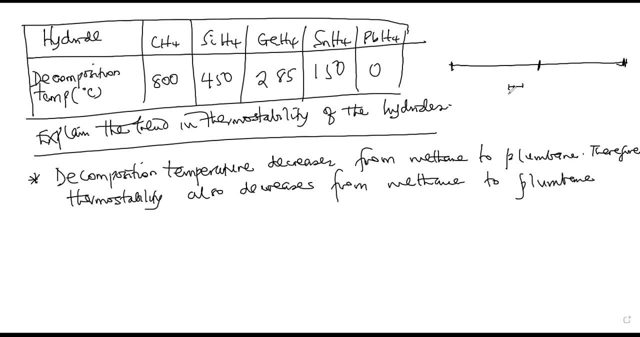 bond strength decreases. that's requiring a decreasing amount of energy to break the increasing we can bonds. so we are generally saying that, uh, this is because you have to give the reason. this is because ironic- radius increases from bonds: carbon for iron, ready for iron, okay, the cup. uh the bond strength, rather the ionic radius increases from carbon for iron. 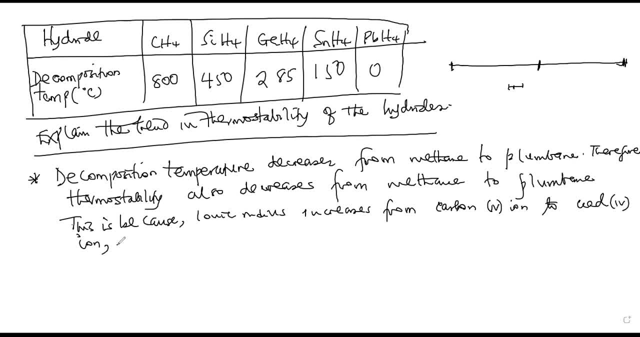 to ready for iron. okay, jewel, perfect now. effective overlapped of the orbitals decreases mm-hmm. the element bond length. the element hydrogen bond length increases. When the bond length increases, bond strength decreases. Bond strength decreases from the bond length From methane to prambene. 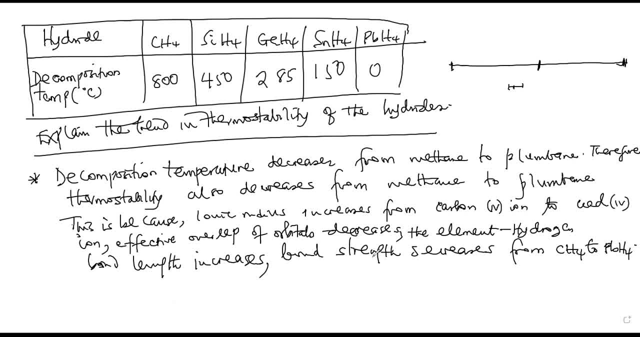 When the bond length decreases, when the bond strength decreases, then it means that the amount of energy required to break the bonds decreases. The amount of energy required to break the bonds decreases. That is it. That is as simple as it is. So that is all about the thermal stability. 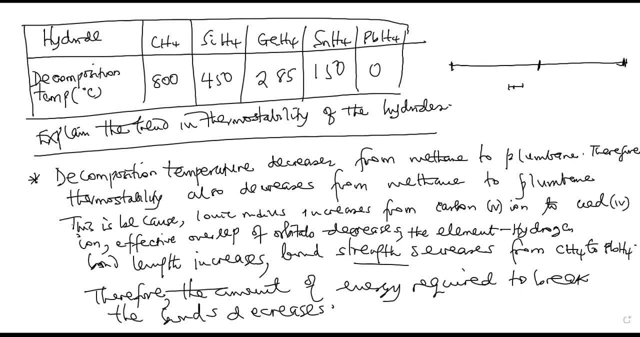 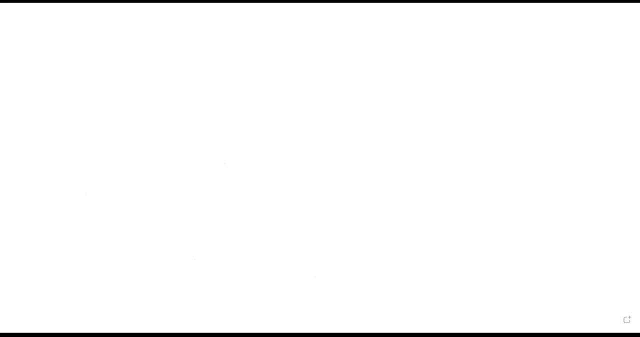 Let's look at how these hydrates undergo Hydrolysis. Let's look at how these hydrates undergo hydrolysis. Okay, Okay, language required to breaking down. Find the Hydrolysis Provide. rights of group four. Provide rights of group four. 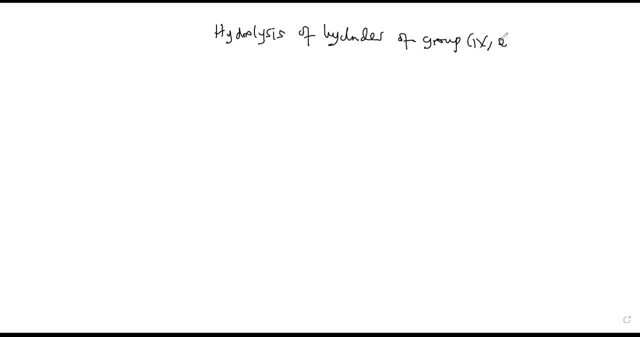 Hydrolysis. So, basically, we are going to find out that siren is the main hydrate that will be undergoing hydrolysis, but we are going to look at under what condition, Because it reacts poorly With water, Others do not, but let's see. 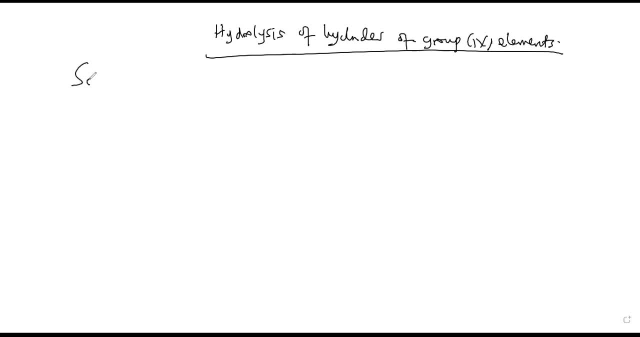 This siren, the silicon hydrate- the one I'm talking about, siren- is poorly hydrolyzed by water, just water. But if that water contains an alkali, Okay, It gets hydrolyzed. Now a question can come. 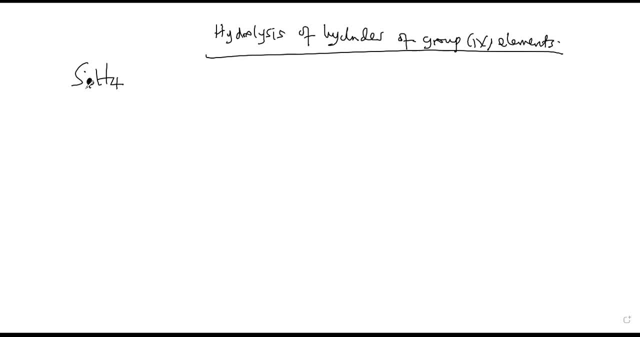 Before we look at it, reacting with the trace, with the water-containing trace of an alkali, or before it gets hydrolyzed with the water, We need to know. We need to know what brings about the fact that siren undergoes hydrolysis but others. 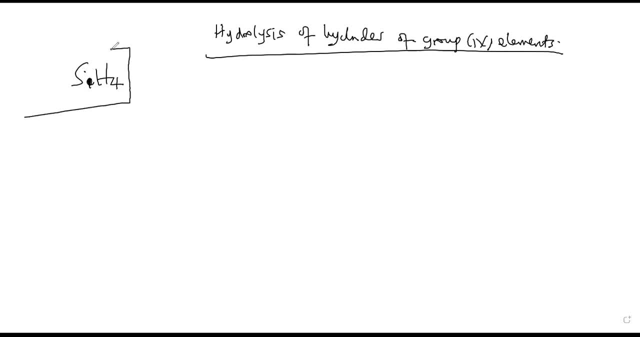 do not. So one can bring you a comparative question. Explain why methane doesn't react with water, but siren does. We know siren Number 14.. the configuration as 1s2, 2s2, 2p6, 3s2, 3p2, 3d0. But carbon 1s2, 2s2, 2p2.. 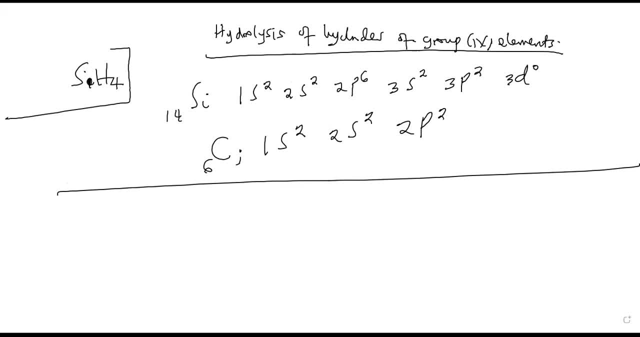 You can really see that the silicon atom in silicon-4 hydride has gotten a 3d orbital, Accommodate the lone pairs of electrons from the oxygen atom in water and thus can undergo hydrolysis easily from silicate ions and hydrogen. So the presence of the empty 3d orbital. 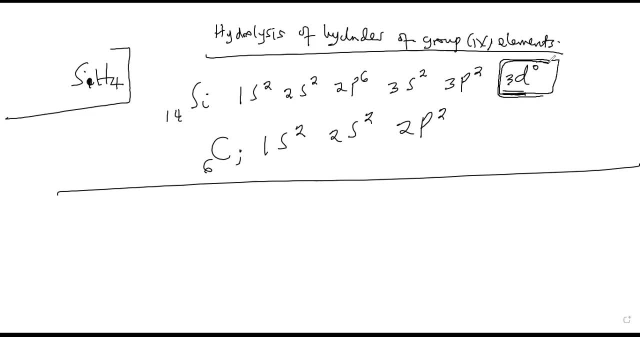 this 3d orbital is received. It is responsible for accommodating the lone pairs of electrons from the oxygen atom of water, Hydrolysis, attracting water. So it attracts water because it has an empty 3d orbital, which carbon lacks. Carbon lacks that empty 3d orbital. 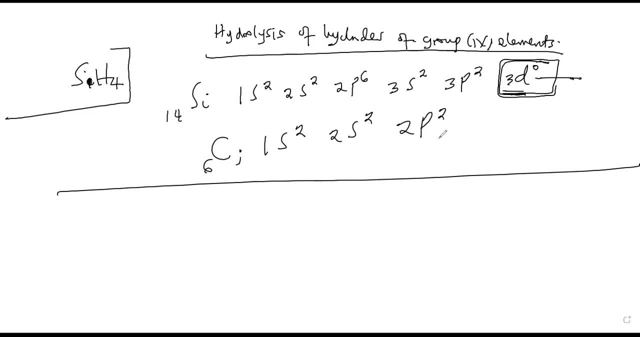 And thus it can not accommodate water. Therefore, it does not undergo hydrolysis. Now, silicon hydride undergoes hydrolysis. All right, It undergoes hydrolysis with water. Okay, It undergoes hydrolysis. 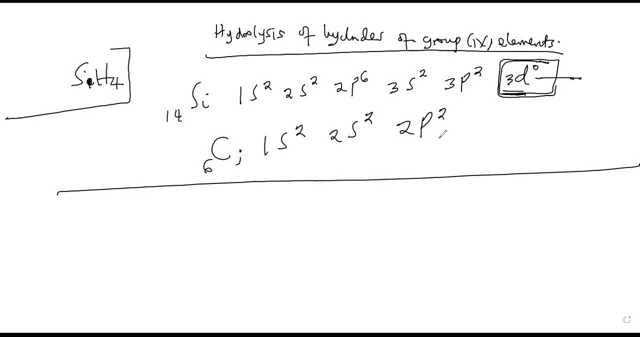 with water, And when it undergoes hydrolysis with water, it forms what we call a silicate. How does the reaction take place? So if they ask you to explain- because now we have already seen the reason as to why it reacts with the 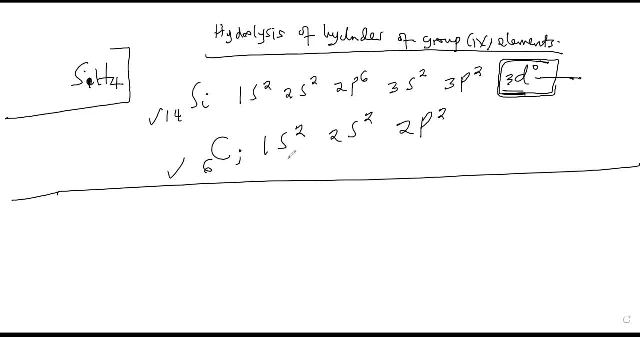 water? why the carbon or other hydrides do not The carbon? it's carbon is lacking the empty 3d orbital. basically, In most of the times the compression is about silicon and carbon. Okay, So this one has the 3d empty orbital that accommodates the lone pair of electrons of oxygen from water. 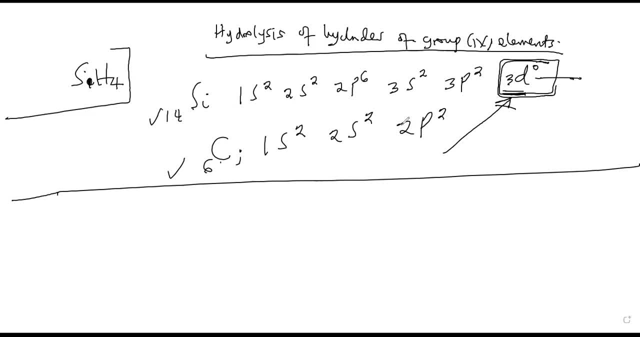 Whereas this one lacks some. therefore, it does not accommodate water and thus can't work, can't undergo hydrolysis. Okay, So if they ask you to uh, uh, exercise, express oxygen, uh, to explain or to describe the reactions of group IV hydrides. 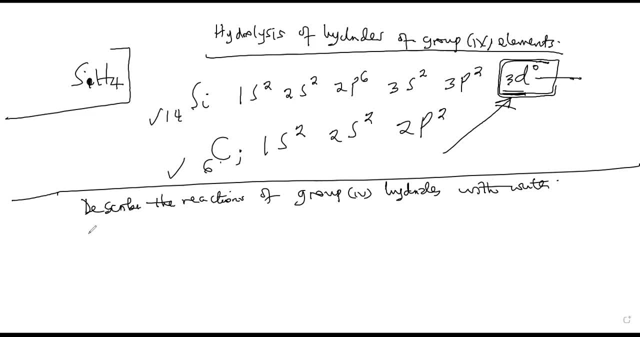 with the water. you have to tell me that siren, because it is only a siren, the rest do not. okay, Methane, gemene, stannane and crumbane, do not react with water. First tell me that statement. 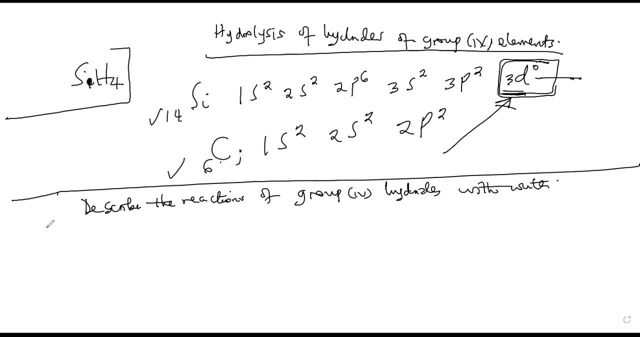 All the others do not react with water, but siren reacts poorly with water to form hydrogen gas and silicic acid, Or one can call it silicon for hydroxide or silicon for hydroxide. You can form silicon for hydroxide. 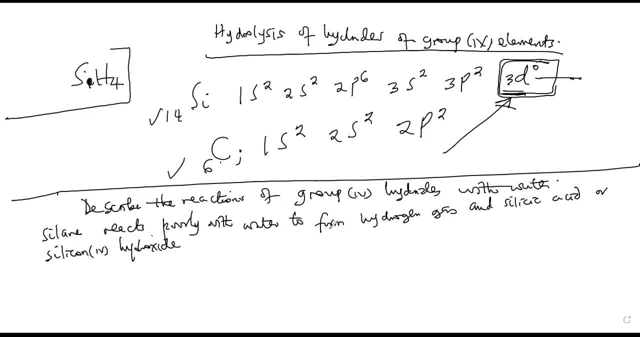 or you can form still hydrated, Hydrated Silicone for hydroxide. Any of these can work. Any of these can work. It reacts with water to form hydrogen gas and silicic acid or silicon hydroxide. 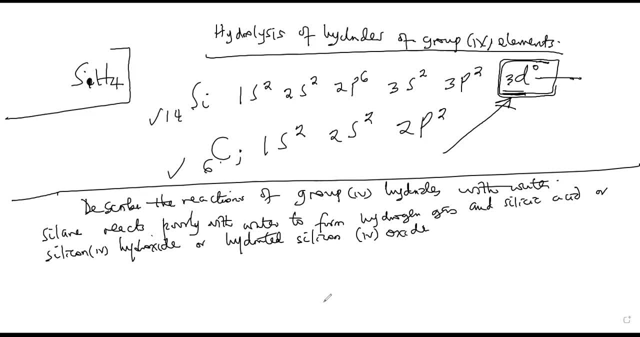 Of course, all of them with hydrogen gas, hydrogen gas, hydrogen gas. So the equations are: you can write silicon hydrogen hydroxide or siren, which is a gas hydrolyzing in water, to form silicic acid. 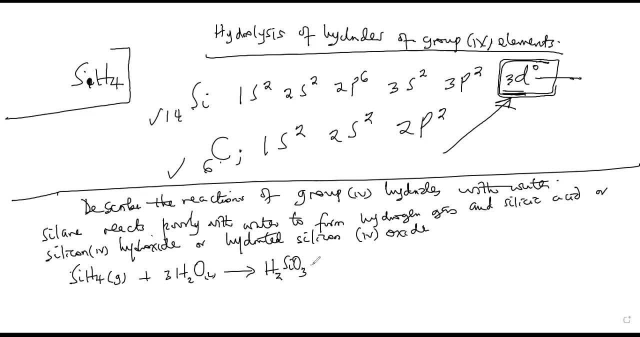 and hydrogen. Or you can write silicon, the reagent for hydrides. you can write silicon covalent and other differentла oxygen, taka sheng. This is how silicon works And this happens. and then 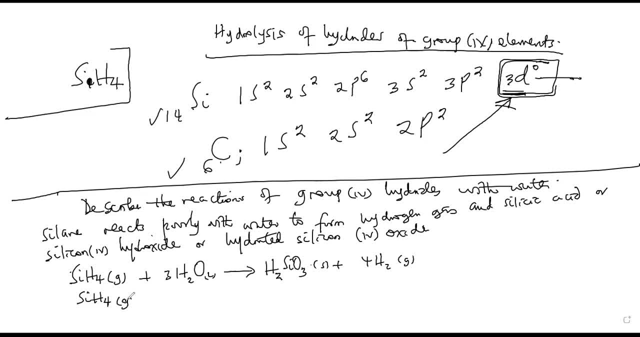 and next and then Siren, and before we have talked about this, this is how silicon works. To form hydrogen. you can have siren, Guan Xilin. that's water. Also put this again: the effect of silicon in water. 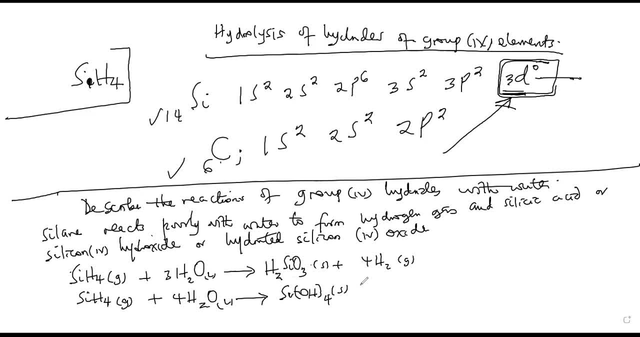 to catch deste plate. So you put silicon here for hydroxide. So if you have hydrogen you can have siren, you can have siren And that has water to come and hydrogen gas. or you can have silicon siren of ours reacting with. 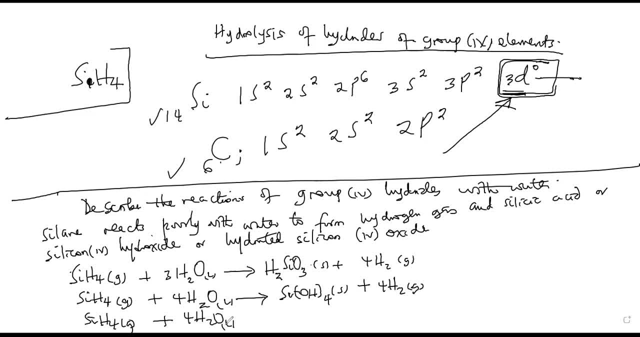 water from hydrated silicon oxide so you can form all these n of those. if the question: you can form n of those, then if the reaction is to be immediate, one can use this, one can explain using this, but after having told me that the other ones do not, or you can bring that statement later. 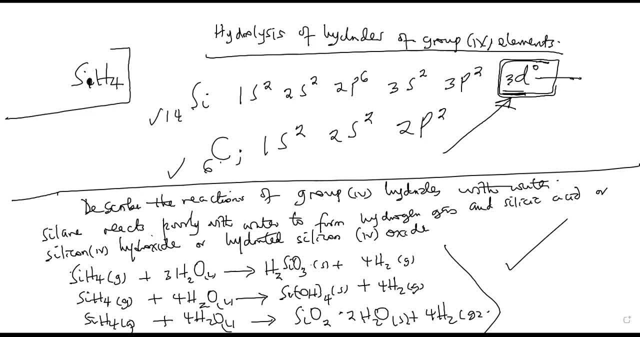 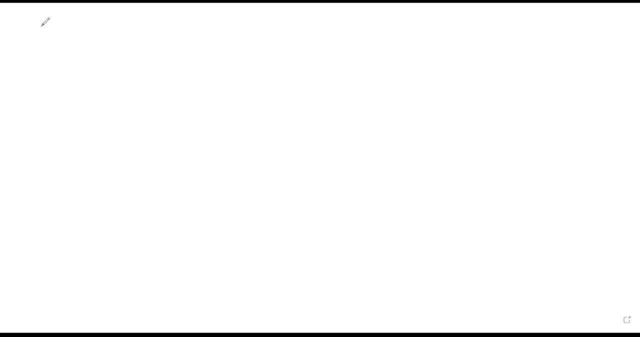 then also we have the fact that, uh, siren also one can say, or not everyone can say- siren reacts with water in presence of, in presence of a trace of alkali, in presence of a trace of alkali, okay to form. uh, what do we form? 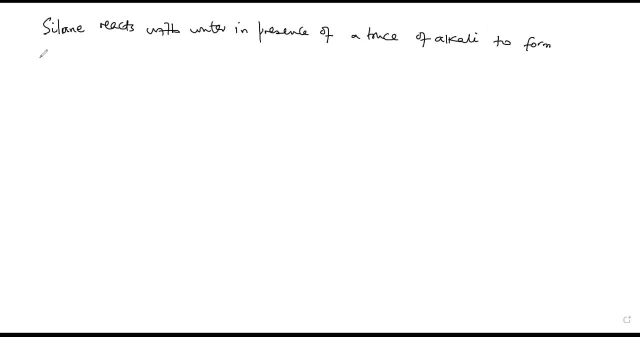 uh, we form silicate ions and hydrogen gas. we form silicate ions. okay, we form silicate ions, where이 before by we shall have siren plus hydroxide plus, as water foam, silicate and hydrogen gas. So that is what we have. 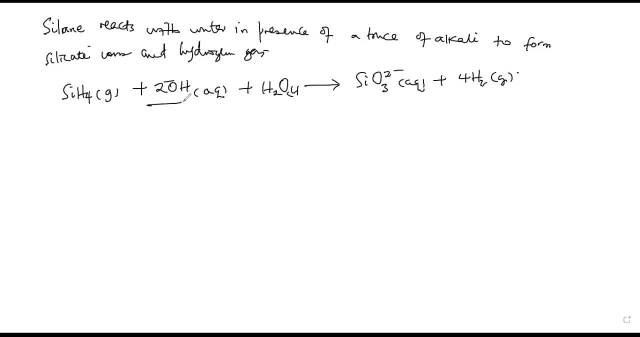 For the reaction to be immediate, we require an alkaline catalyst. Basically, the reason is because the silicon hydrogen bond is less polar, simply because these ones have got almost equal electronegativity. All the electronegativities are almost equal. 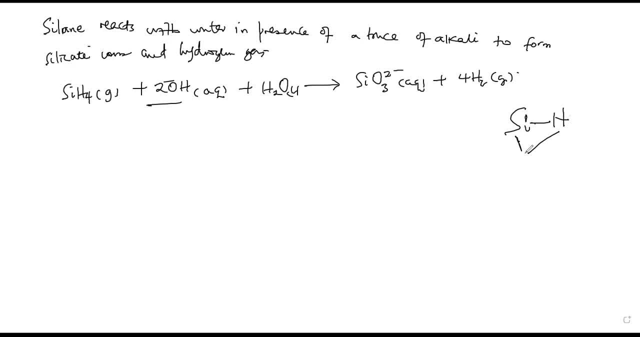 And therefore they are less polar. The bond is less polar. If the bond is to be polar, that means that there is a big difference in electronegativities, But because the electronegativity of silicon is almost the same as that one of hydrogen. 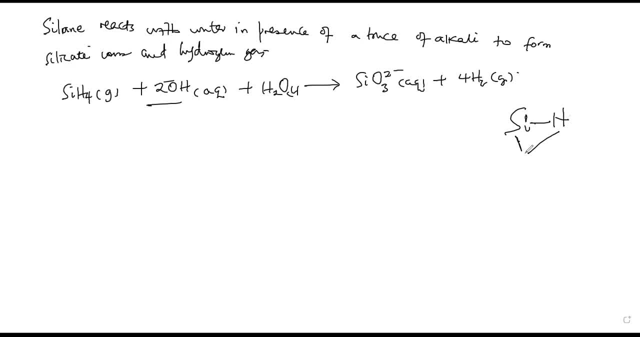 then the bond is less polar. So that is what we are having, But the rest do not react with alkaline, Even if the question is not. rather, do not react with what, even if the question is very changing. to what? These hydrides, apart from the one of silicon, the silane? 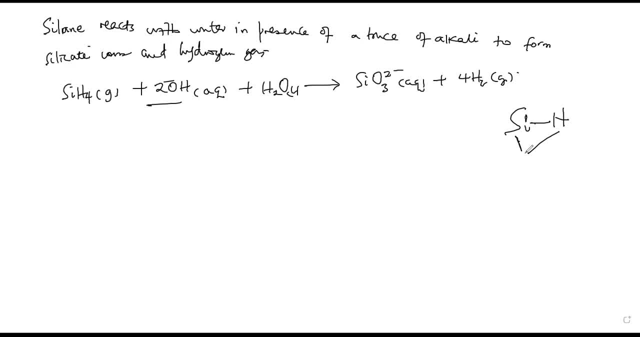 the rest, do not react with it, with the water, OK. so, members, from here there comes a question. Let's look at how these hydrides react with acids and alkalines. Reactions of these alkali, of these hydrides. 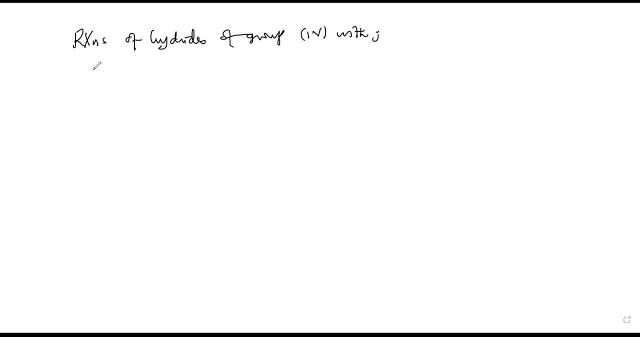 With the acids, And two acids, alkalines. The fact is these, these hydrates, do not react with with acids. All right, They do not react with with acids. So if the question is: last year they tricked students. they told them to describe 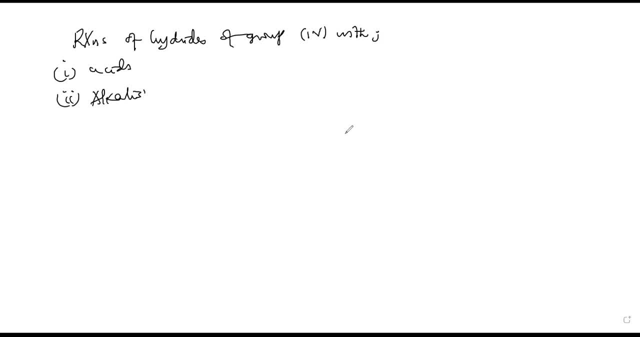 how the hydrates react with the hydrochloric acid, and they put two and a half marks. A student just says silicon, silicon, do not react with the acid specified. You will get your two, two and a half marks, But they put two and a half marks. 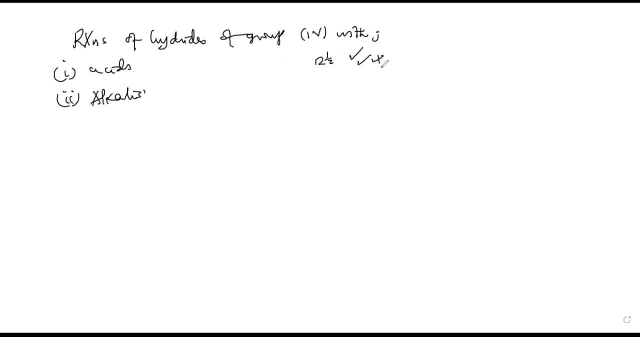 and the student starts thinking, okay, don't overthink. Okay, now here with acids for Roman one. you just need to know that the hydrates do not react with the acids, With the alkaline or what. Ah, The marks put there, you can't fit all of them. 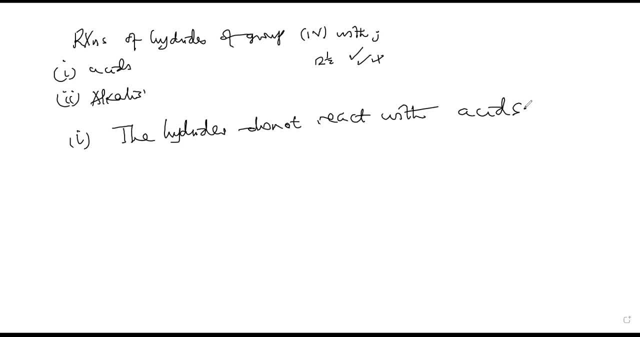 as I've told you. Then with alkalines: reactions with alkalines: methane, germane, stannate and plambane do not react with alkalines. Okay, You first need to specify the other ones: methane, stannate, germane and plambane. 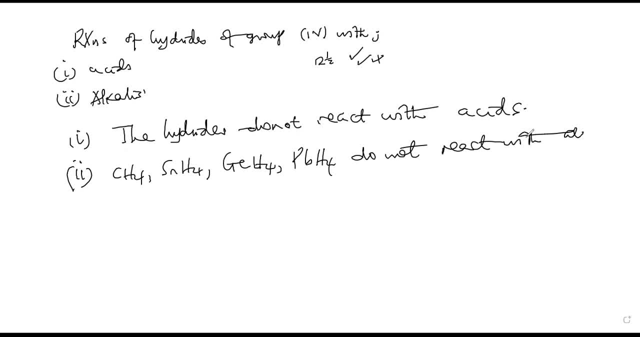 do not react with alkalines, Okay, But Ah, simply, what happens Is that On received, Okay, On received, we react with the sodium hydroxide solution or acquiesces sodium hydroxide From sodium hydroxide. it's not, It's just%. 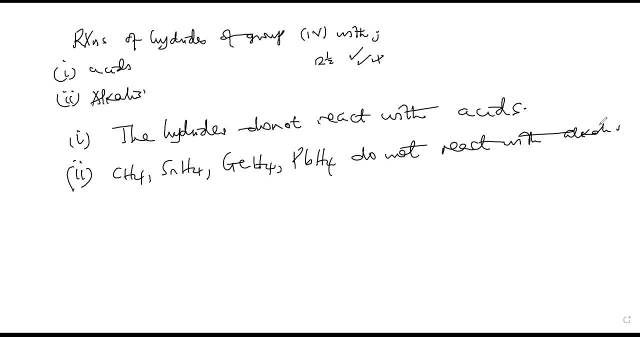 from sodium silicate or from the silicate ions and hydrogen gas. so here we shall quote and say that silane, since they have not specified which alkali, so cyan reacts with the aqueous alkalis, okay, to form the silicate ions and hydrogen gas. how we shall have silane. 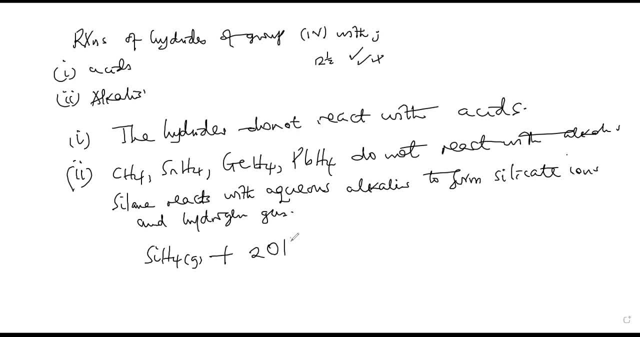 reacting with the aqueous alkalis. as i have added water up here circle, i appears aqua water to form a silicate ion and hydrogen gas. so this is what we have. okay, so basically that's what we have. and here you have the NZD water. okay, so basically that's what we have. 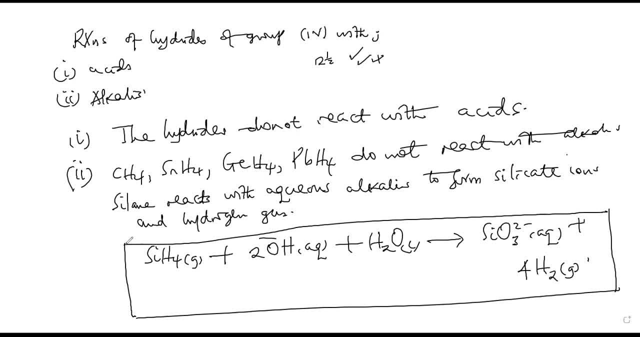 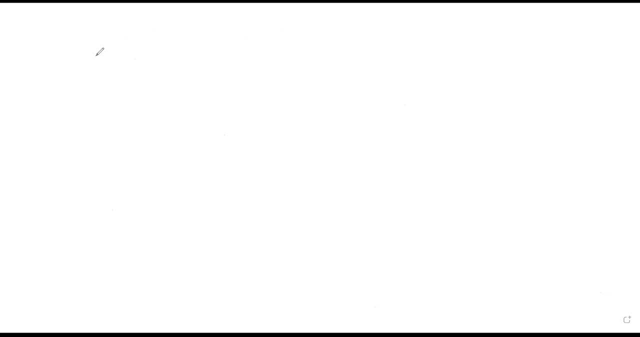 that is how these substances react. okay, Then let's look at how they burn in air, And this is my last part. Burning in air: how do they burn in air? Combustion, Combustion. Let me first outline for you the equations. 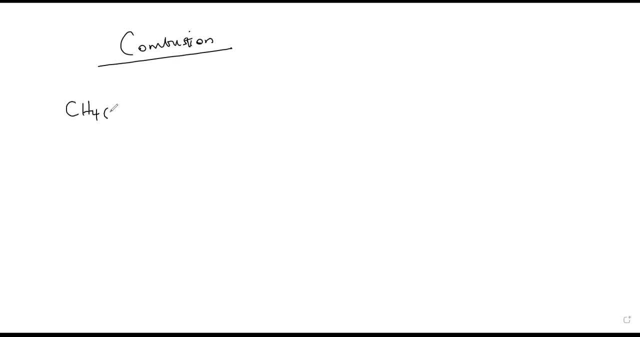 Methane. from organic chemistry we know that it burns in oxygen from carbon dioxide. They form dioxides, apart from lead, which forms a monoxide. So this one forms carbon dioxide and water. Siren burns in oxygen from silicon dioxide and water. 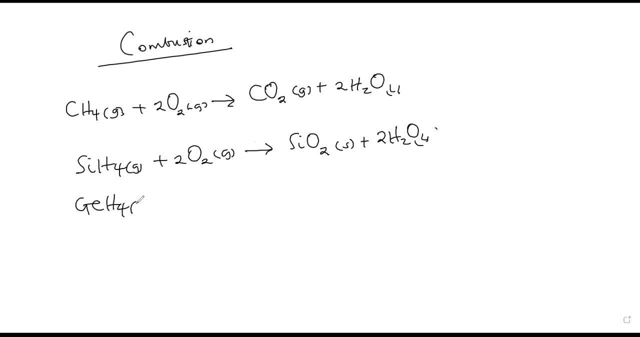 Germain burns in oxygen from silicon dioxide and water. Tin burns in oxygen from germanium and water. Tin burns in oxygen to form tin. Siren burns in oxygen to form tin. Ramban burns in oxygen from lead to oxide and water. 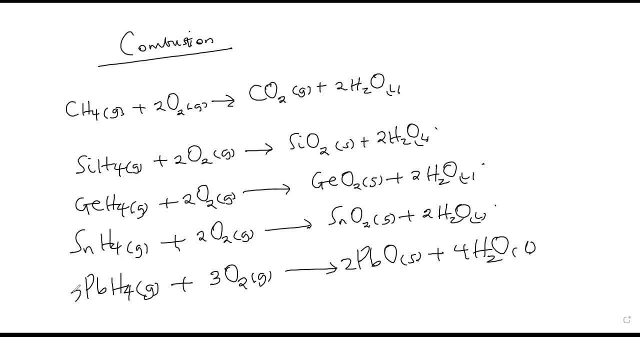 Here we have that too. Here we have that too. So one can already say for this the reaction: methane burns in air at higher temperatures or temperatures above like 500 to form carbon dioxide and water. Siren burns, this one burns spontaneously. 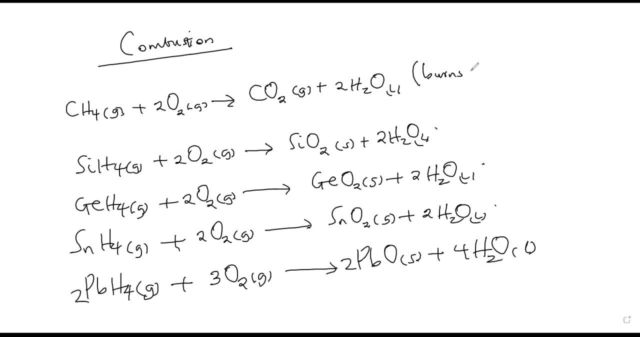 Siren burns at temperatures above 500 degrees to form carbon dioxide and water. Siren burns spontaneously. Siren burns spontaneously from silicon dioxide and water. Ramban burns in air at intermediate temperatures, But with these ones they burn in air direct to form this one forms tin oxide. 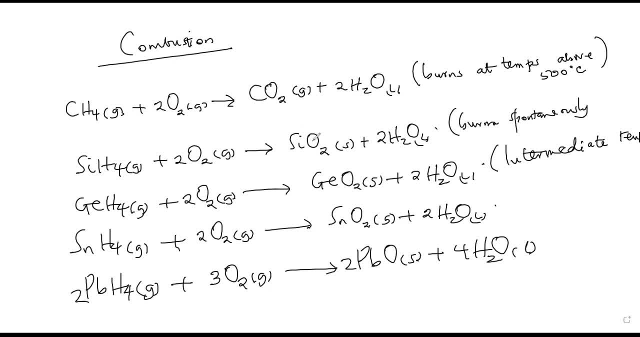 This one forms lead oxide. Here we formed germanium oxide, Silicon oxide, Carbon dioxide or carbon dioxide. So this is how these hydrides burn in air. For your own information, this question appeared and let me look at the version. the question that appeared in last year's UN. 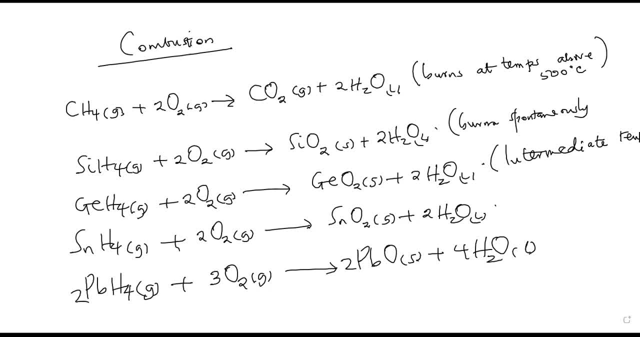 And this one has called us to come to the end, Or it will call us to come to the end of this topic. But that is after having done some of the questions, Some of the questions. So the rest of the work, we have already looked at it. 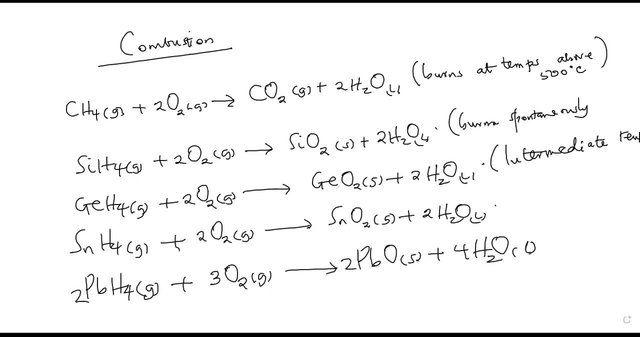 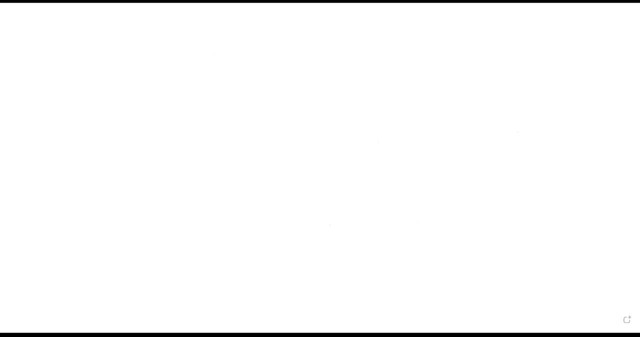 And it is being uploaded, The rest of the work about group four elements. So it is all ready. But let's look at the sample question about hydrides, as I have already done. They say that carbon, silicon, tin and lead are some of the elements in group four of the periodic table. 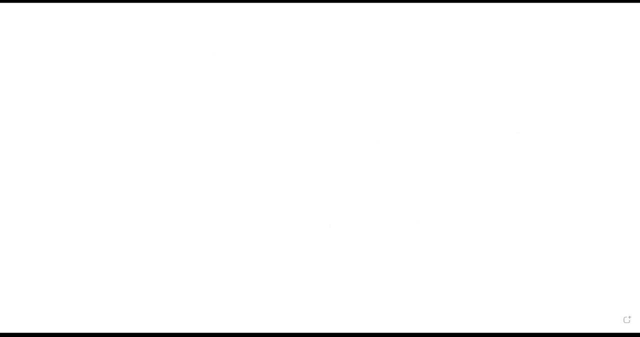 Write the formulae of the hydrides. Just writing the formulae of the hydrides. Was taking marks, Was taking marks. Then they went ahead and said that carbon can combine. This question was the one which was a bit. Carbon can combine with hydrogen to form a wide variety of compounds. 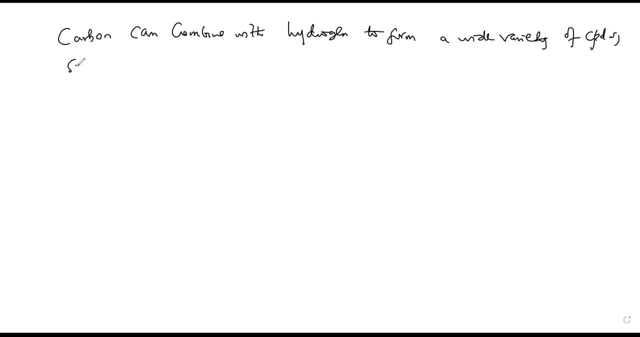 Carbon can combine with hydrogen to form a wide variety of compounds. Silicon Forms fewer Compounds With hydrogen, While While Hydrogen Compounds Of lead And tin are very limited In a number. Explain: They gave it two marks. 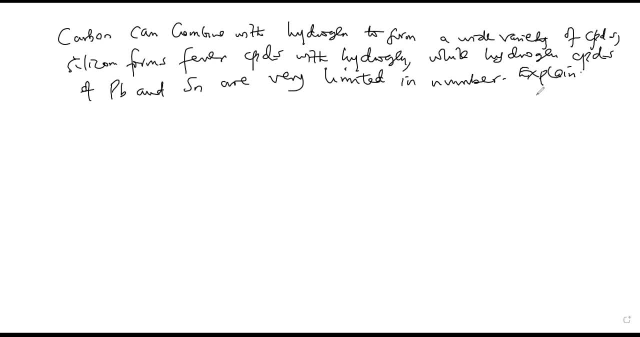 They gave it two marks. Explain They gave it two marks. They gave it two marks. This is Why- Why carbon forms variety. Silicon forms fewer, While lead and tin, Tin, Rather, Form fewer. You need to know that the reason as to why carbon forms the 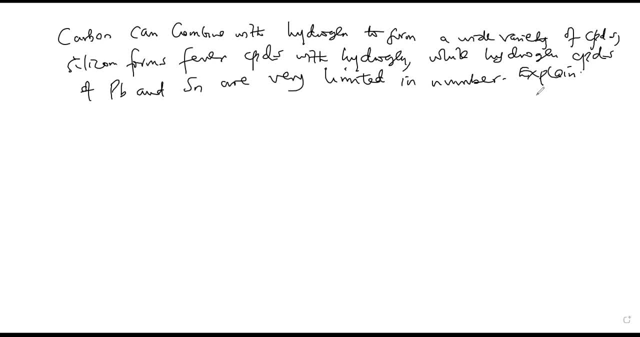 The variety Of compounds with the hydrogen. The whole aspect is catenation. Carbon undergoes catenation. When we say catenation, we are trying to talk about forming long chains or rings, Or one can say forms stable multiple bond. 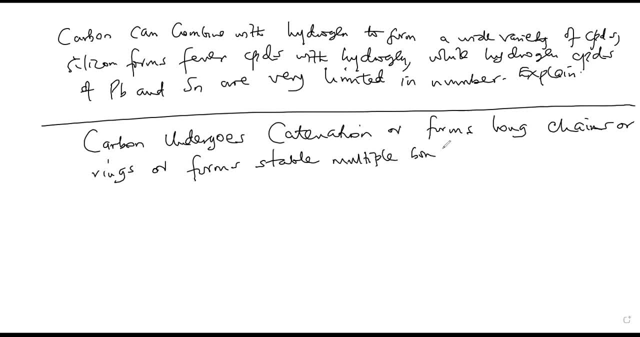 A stable multiple bond with itself and hydrogen With itself and hydrogen. The aspect of catenation was covered in lesson one of this thing. It forms stable multiple bonds with itself and hydrogen And down the group, down the group, atomic radius increases. 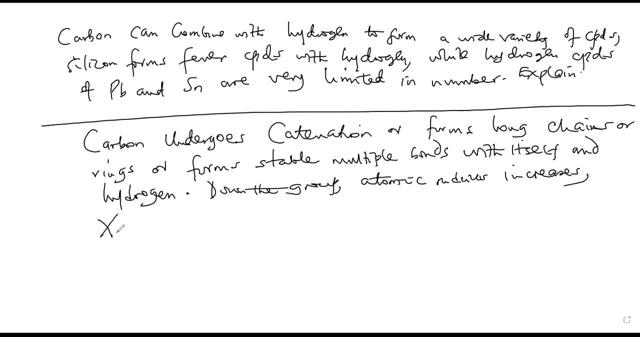 And x hydrogen- meaning x can stand for any atom- becomes longer and less stable. So we are bringing in the aspect of stability, We are bringing in the aspect of what, what brings in the stability, We are bringing in the aspect of catenation. 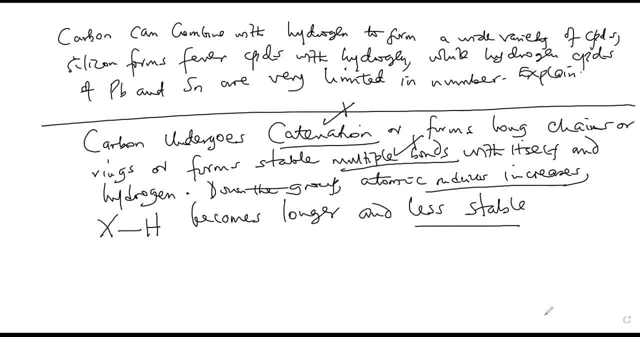 So it undergoes catenation or it forms multiple bonds with itself and hydrogen, Unlike others. more so, the atomic radius increases down the group, making this hydride become longer and weaker and thus less stable. So that is the reason as to why carbon forms. 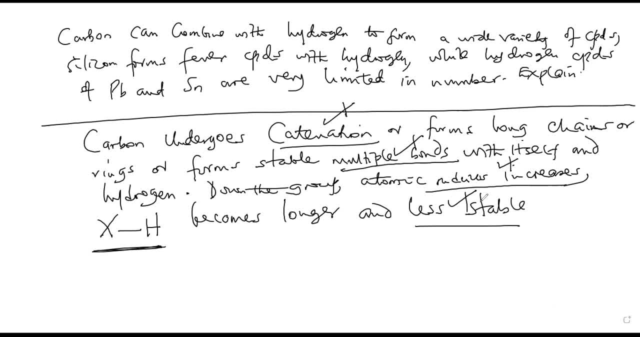 why the variety of compounds unlike others? Okay, So then from there, from there also, we need to know. we need to know that still more so as it does this. Anyway, that was part two of the question. I think I can't add on anything on this. 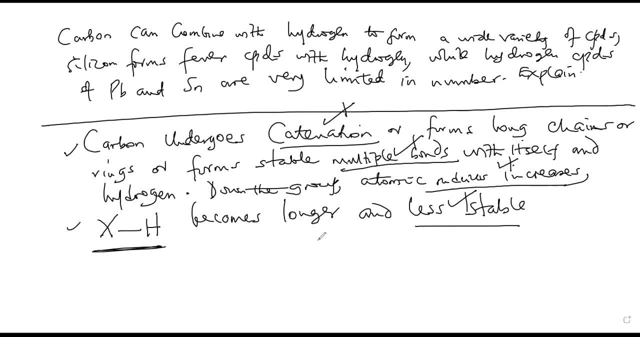 That is part two of the question. Then part C. they wanted students to discuss the reactions of hydrides with the dilute hydrochloric acid, Reactions with the dilute hydrochloric acid, and they gave it two and a half marks. 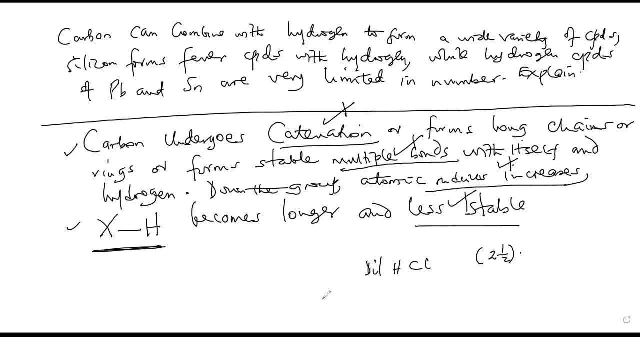 A student would just say: the hydrides do not react with the dilute hydrochloric acid. And the guide was saying: give two and a half Because they don't react with the acids, Then with the sodium hydroxide, of course. 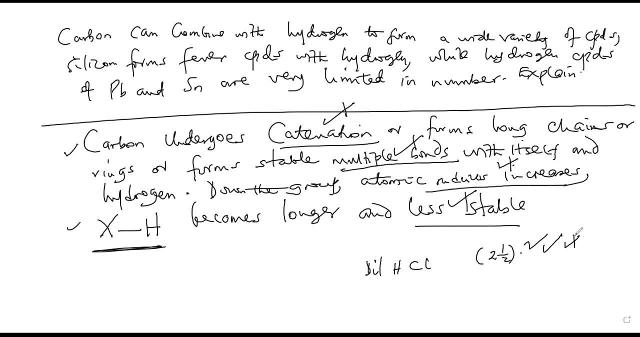 you talk about siren only the way we have done. Then with water. still you talk about siren only with all we have done. They were given two, two marks, So the student there would fit six and a half marks on that reaction. 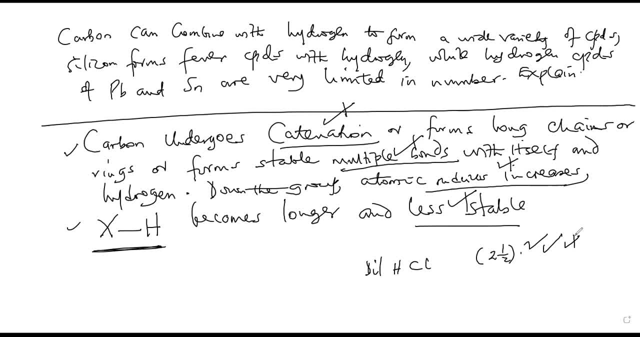 two marks on the right on writing the hydrides and two marks on explaining this. Okay, Then there was a question of explaining how chlorine reacts with the tin and lead. How chlorine reacts with the tin and lead, much as we have covered it at the starting. 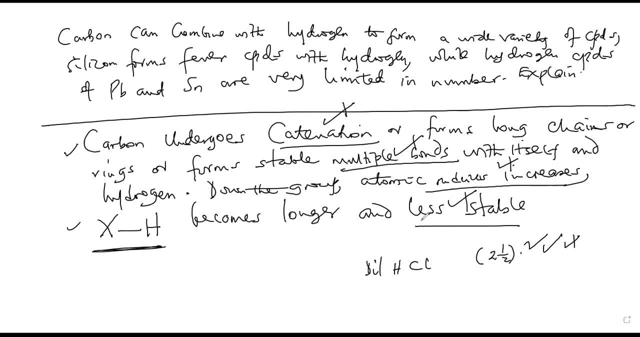 how chlorine reacts with the tin and lead. We already covered it in the first, in the first place. Okay, Actually, that was the first video. Okay, How chlorine: describe- explain how chlorine reacts with the tin and lead. For Max: 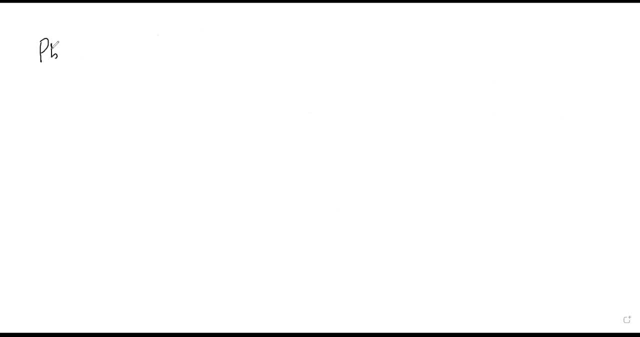 Tin and lead. Tin and lead- This is lead And this is tin. Need to first know the equations. So tin reacts with the chlorine to form tin folcloride Liquid. So if you were to explain, they want to explain how tin reacts with the chlorine. 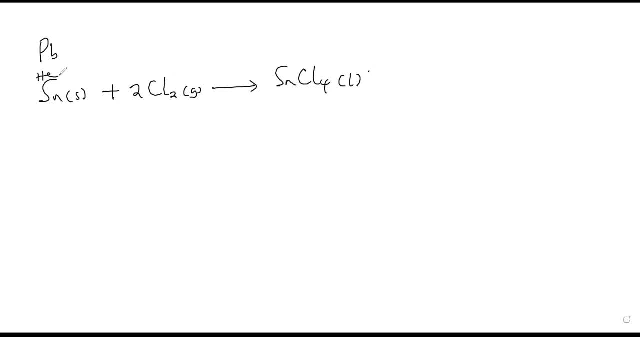 So you first tell me that heated tin must be heated. Heated tin reacts with which kind of chlorine? Reacts with dry chlorine. Reacts with dry chlorine to form tin, folcloride, Form tin folcloride, Heated tin. 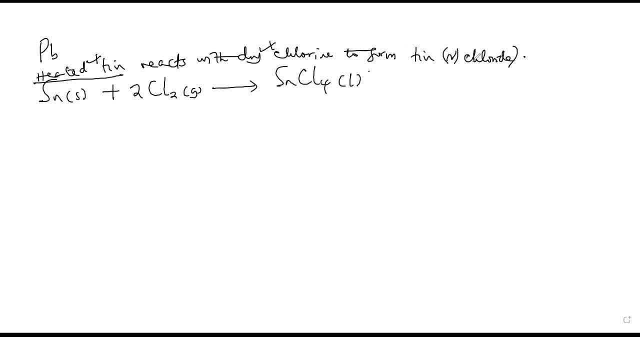 reacts with dry chlorine to form tin folcloride And that is to Max. For lead, it is heated lead. The same way reacts with the chlorine, But for lead. we don't form lead for chloride, but instead we form lead to chloride. 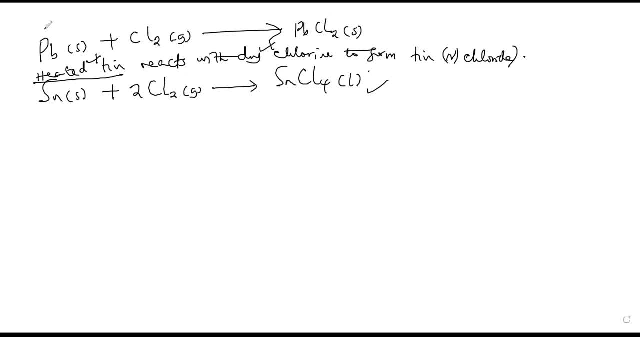 And lead to chloride is a solid, So you would say lead. heated lead reacts with dry chlorine to form lead to chloride And this was manifested, why we form lead to chloride. We manifested it when we started the stability of the chlorides. 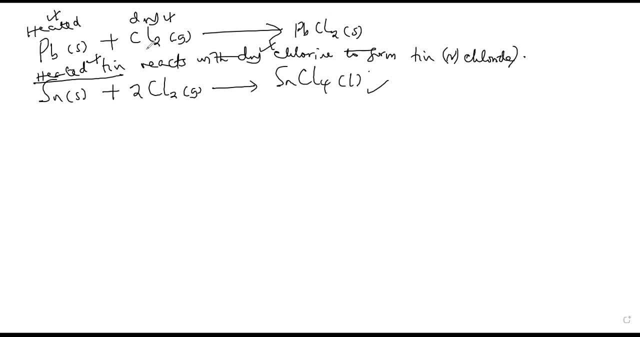 of these, of these elements, All right. So where we looked at the stability of the dichlorides For this case, for this case, we shall have some when those when you review the work that we first uploaded for dichlorides. 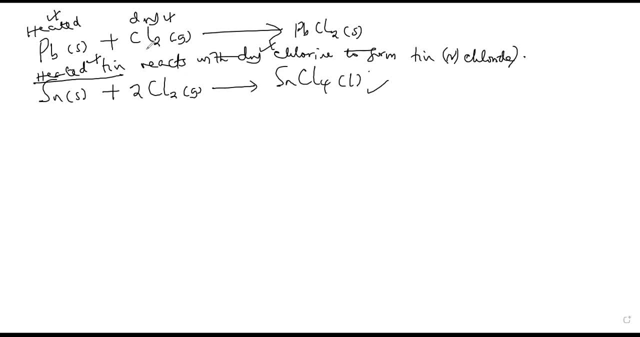 the oxide. you are willing to understand deeply the issue of the oxidation states and rather the stability of these compounds. So those who are taking four marks students made a mistake by saying that lead also forms lead for chloride. That is. that was wrong. 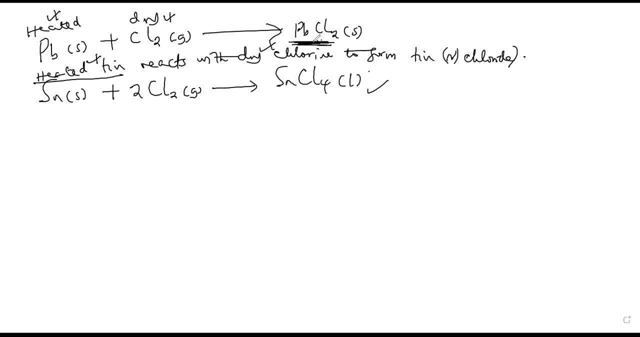 Then another reaction was nitric. how nitric acid reacts with the carbon and lead. That was taking five and a half. How nitric acid reacts with the carbon and lead, Of course, of course you need, what you need to really know is that. 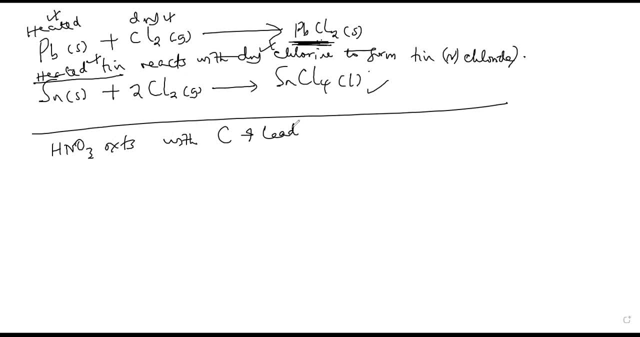 nitric acid if it is dilute, if it is dilute nitric acid, dilute nitric acid to react with the. it does not react with the carbon. That is what we need to really, really, really understand. Dilute nitric acid does not react with the carbon. 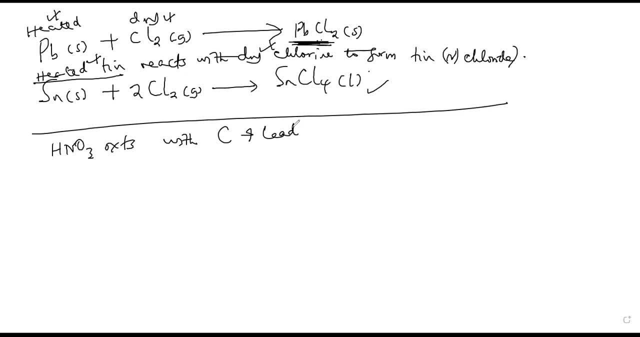 But concentrated nitric acid acts as an oxidizing agent and it oxidizes, oxidizes carbon. Okay, So one will tell me that concentrated, or you can say that carbon is oxidized by hot concentrated nitric acid. Then you have to write words. 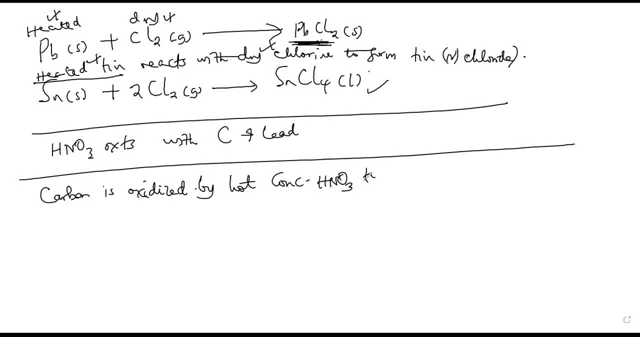 what concentrated nitric acid to carbon dioxide. carbon dioxide gas? of course, nitrogen dioxide gas and water. Of course you have to write words, Then you have to write the equation for the reaction. Carbon dioxide is oxidized by hot. 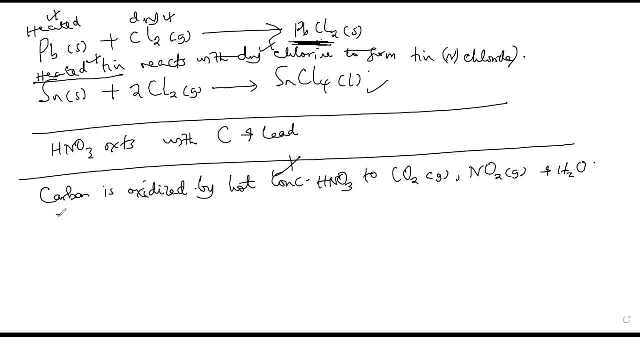 Then you have to write that Equation. So it is carbon solid plus hot cong. Hot cong, That is for molecules of nitric acid and is oxidized to carbon dioxide. Then the nitric acid itself is reduced to nitrogen monoxide. 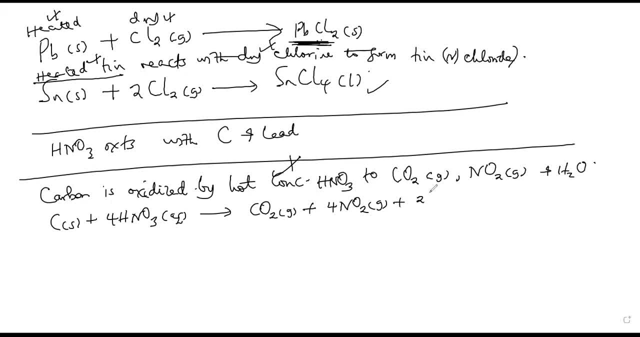 rather nitrogen dioxide and water. All right, So carbon is oxidized by hot nitric acid to carbon dioxide. Then here you get your marks. Then lead. For the case of lead, you can write a series of ideas which can be accepted. 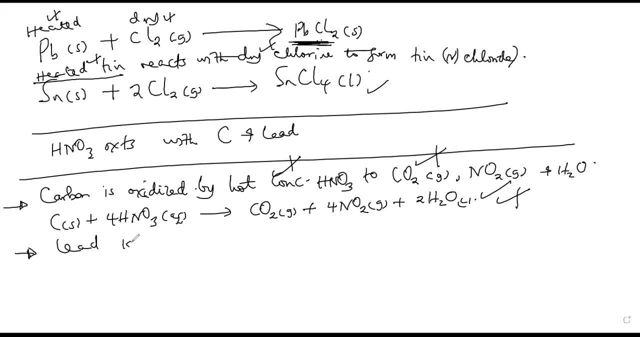 That is for carbon, But for lead is oxidized by hot- All right Hot. Or one can use warm concentrated nitric acid to form lead to nitrate. So here you have nitrogen dioxide. Those are two words, Nitrogen. 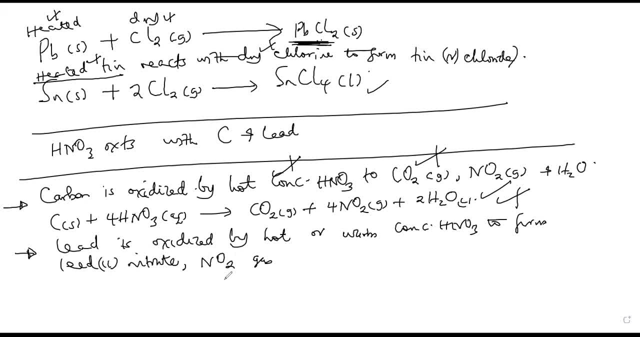 Then dioxide, Gas, All right, And water. So here one can write: lead plus four molecules of nitric acid appears to form lead to nitrate, And here you have the two words Acquiesce, Acquiesce And. 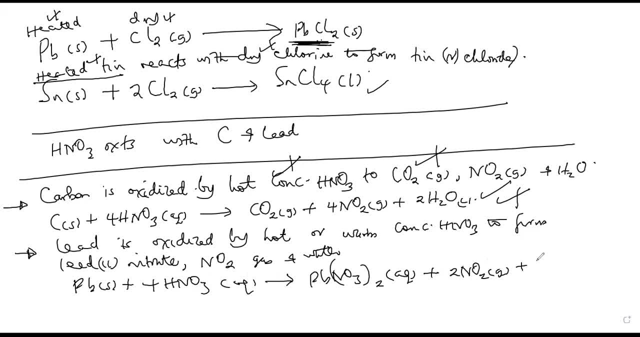 nitrogen dioxide, Gas, Then water. So that is the aspect of lead. Or here you're going to get all your marks- One and a half, Hot or warm, from lead to nitrate. Okay, Then one can say for the case of lead, 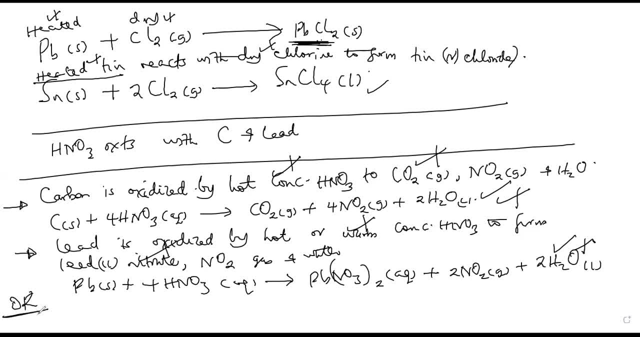 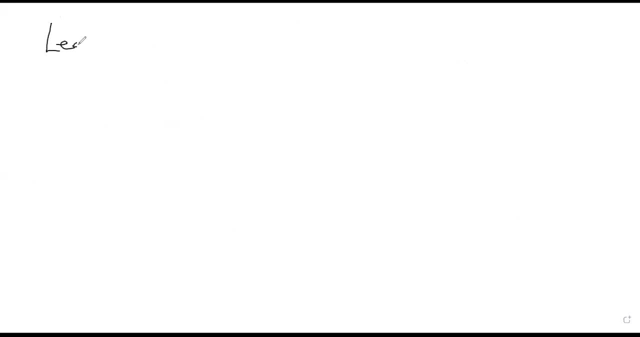 one still can say lead reacts with warm or hot or hot moderately concentrated acid. Okay, All these ones were awarded. One can say lead reacts with. the lead reacts with warm or hot, moderately hot modality and pump moderate nitric acid still to form.